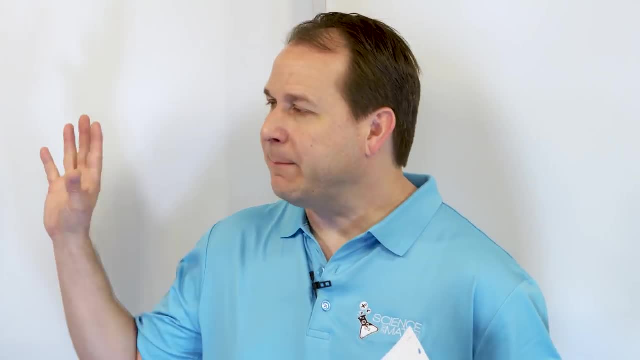 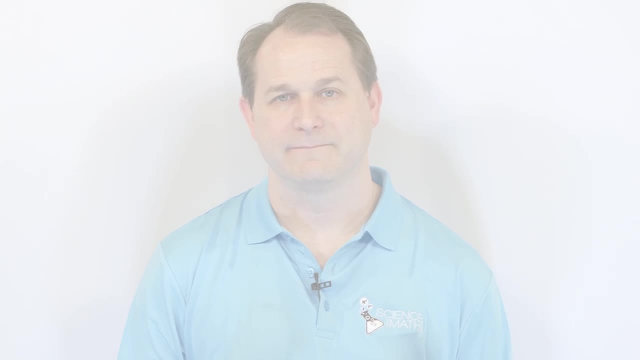 and the quartic equations, which is the power of four. So before we get back to the board here, let's do that computer demo And I'll show you graphically what the roots of these different kinds of equations really look like. Okay, welcome back here. What we have here is a little demo that. 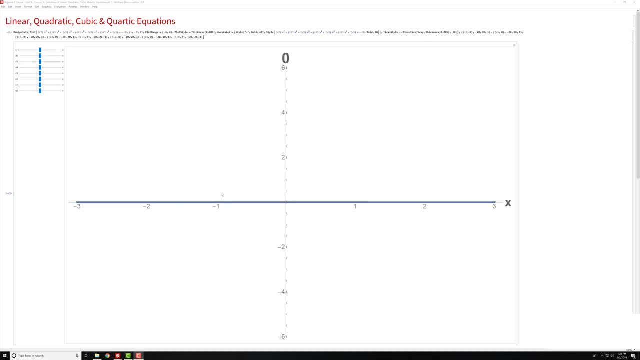 I've done. here I can show you the different graphs of the different kinds of equations. here We have linear equations and the higher order polynomials beyond that. So the simplest kind of equation you can have is a horizontal line. So the graph here it just says three. here That means y equals three. 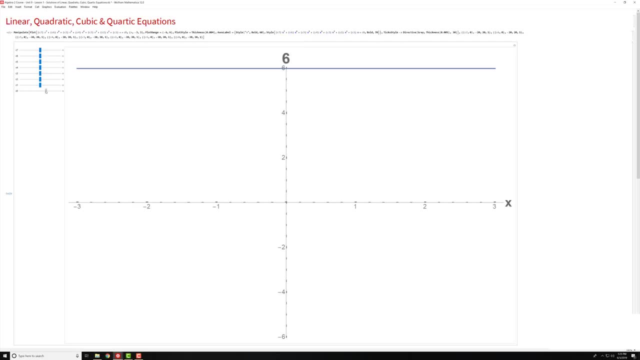 That's a horizontal line that crosses it at the value of y is equal to three. Here the line crosses at the value of y is equal to four. You can see that this horizontal line does not cross the x-axis at the x-axis at all, So it doesn't have any roots. But if we make the line a little, 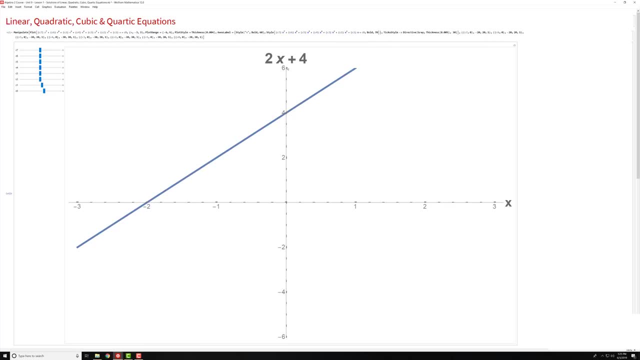 more interesting. we can see that the x-axis does not cross the x-axis at all, So it doesn't have any roots. So it's just a little bit more interesting If we put a slant to it. then here is the equation. 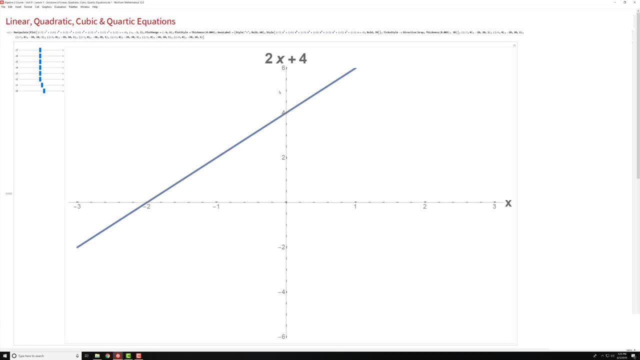 of this line, two x plus four. You can see the y-intercept is up here at four and it has a slope of two rise over run. That's what this means. right, And you can see that in general, when a 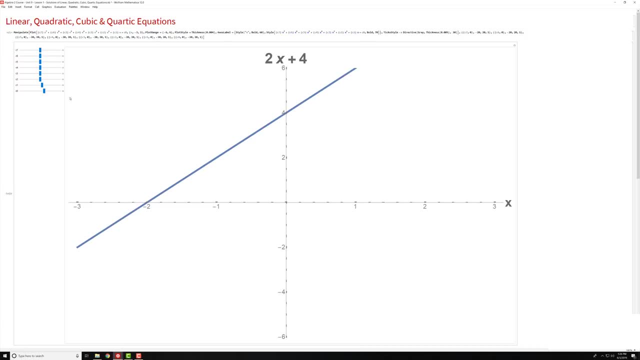 line is slanted, it is going to cross the x-axis in one location. Now I can play around with this line. I can bring it down like this: So the y-intercept is negative. three down here And you can see that the root here of this first order equation, see the power of x. here is just a one. 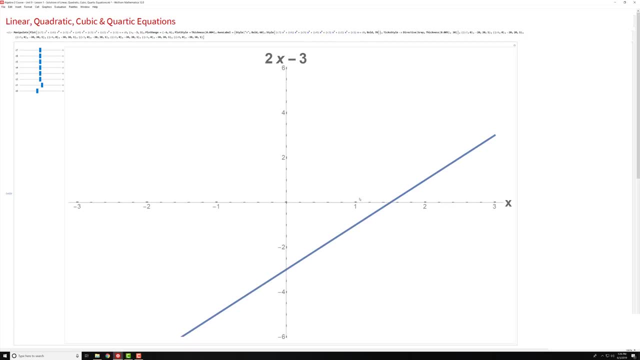 So we have a first order root here, which basically means we expect to have one solution when we set this guy equal to zero, which means one crossing point. Here's the crossing point. Now, no matter what I do, even if I make the line slant the other direction, if I shift it up or down, basically move the line. 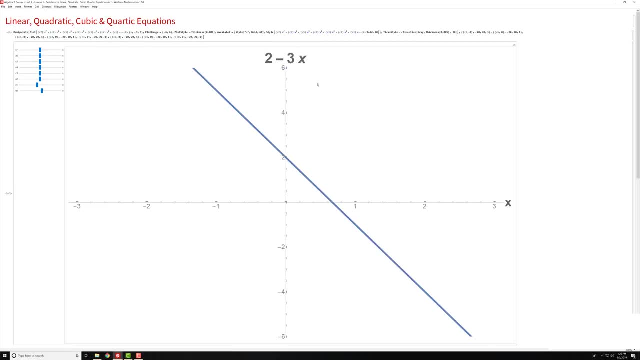 around. it's only going to cross the x-axis in one location. It has one root, because the power of x is just a number one. Now let's go up and I'm going to drag my slider here to make a quadratic. So this is a simple quadratic and I can reset the rest of these guys here to kind of reset. 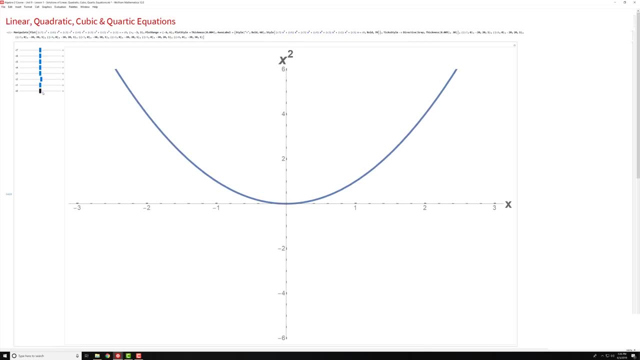 what I have here. So this is the quadratic: y is equal to x squared. If I change it to make it, for instance, x squared minus three. this is what this curve looks like Now. the highest power of x here is a two. That means it's a quadratic. All quadratics have a power of two for the highest. 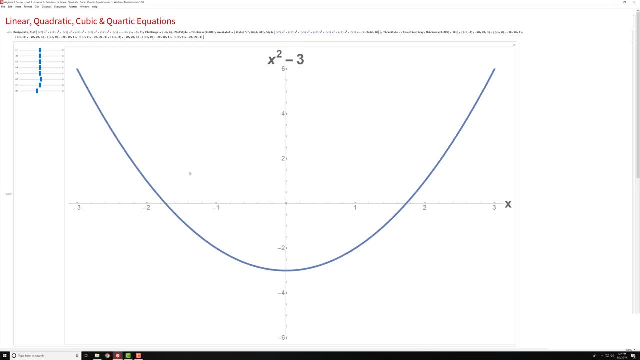 power, And because the power is two, that means that we have two roots of this equation, right? In this case, one root is where it crosses the x-axis here, and the other root is where it crosses the x-axis here. So this is a simple quadratic and I can reset the rest of these guys here to kind of. 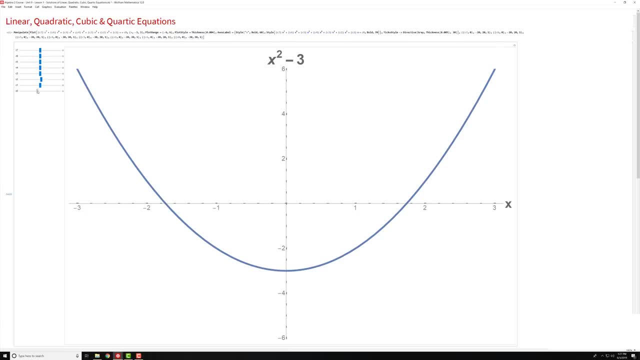 the axis over here, So you can see that there are mirror images. Now, as I change the graph a little bit, you can see the crossing points are in different locations, but they're still two roots. Now, if I change very slightly what the equation looks like, maybe make the parabola more sharp by 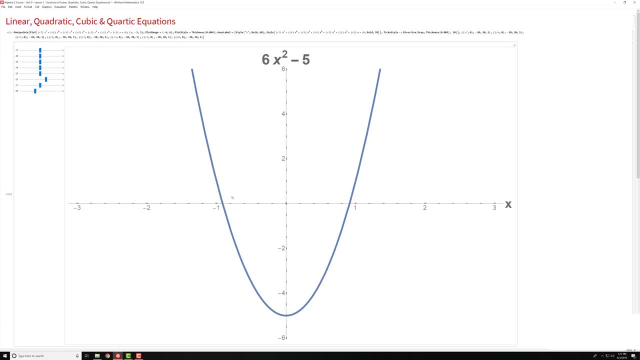 putting a higher coefficient in front of the x squared. here it does change the shape of the curve, but we still have two crossing points. And with quadratics we have always expect to have two crossing points, because the highest power of x is a two, Just like in the case of a line. 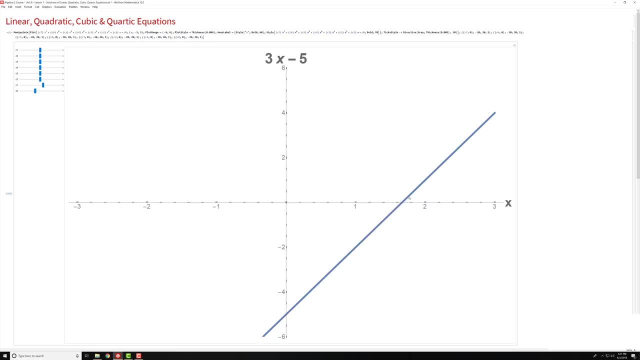 like this line right here, or any line in general, we always expect only one crossing point, because the highest power of x is a one here. So let's go back up and make it a quadratic. Now you can see we have two crossing points. You can see there's a crossing point here. there's a crossing point. 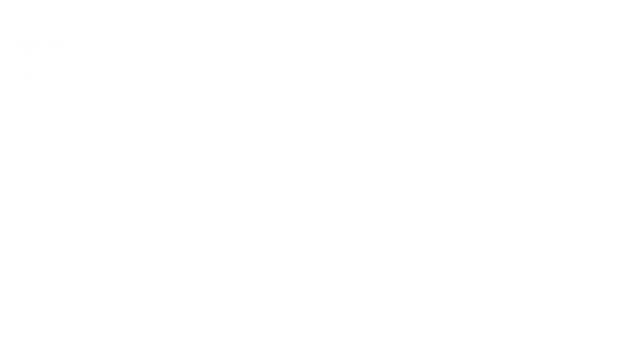 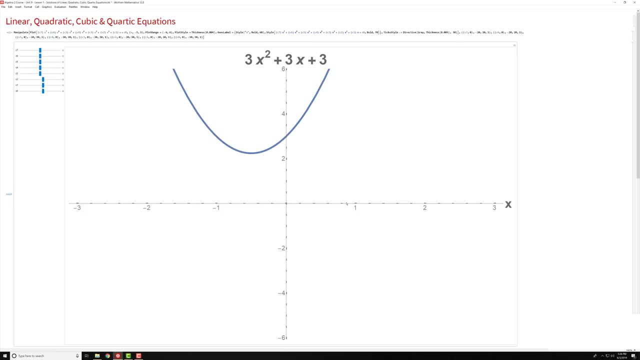 here. So we have two roots. Now, what I want to draw your attention to is, if I drag this quadratic above the x-axis so that you see how it never intersects, this quadratic never intersects the x-axis at all. That means that this function never, ever, has a value where it's equal to zero. 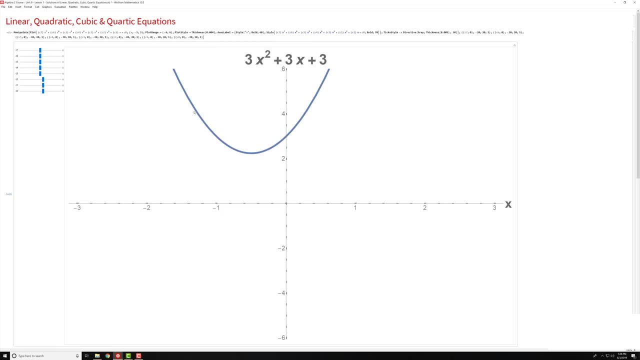 So it doesn't have any real roots. But, as we're going to learn here very soon, when we talk about the quadratic formula, we're going to see that this quadratic equation still has two roots, but because we don't have any crossings on the x-axis, they're not real roots. We always have two roots, but it's going to. 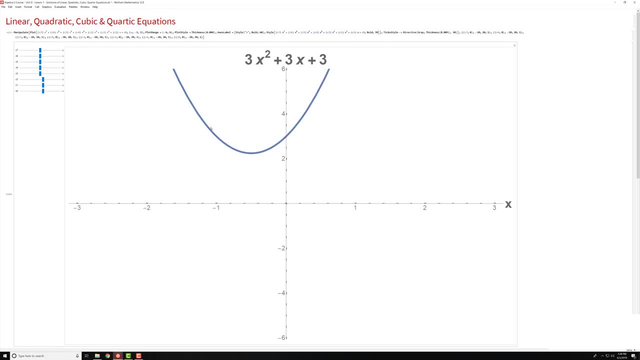 turn. we're going to turn out and see that when the graph is floating up here, we have two complex roots, or imaginary roots. We've talked about complex numbers before, So this quadratic equation still has two roots. It's just that they're both complex And so we can't see them on this graph of. 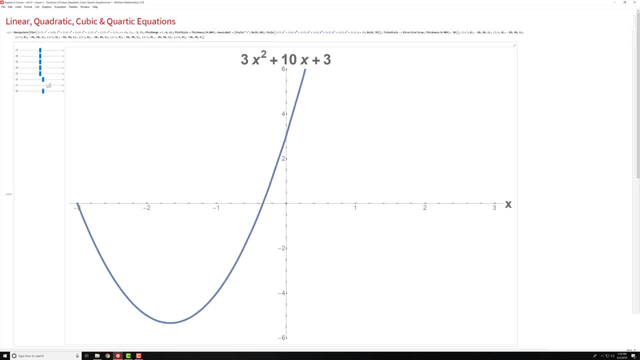 real numbers, the x and y graph here. So you see, no matter what I do, if I move this guy, maybe over here, maybe shift it way up high. you see down below. once it crosses down below, we have two. 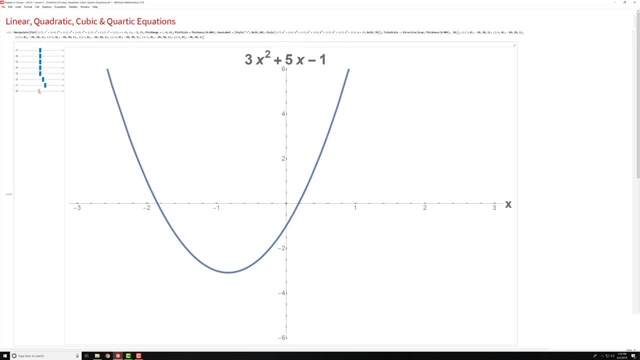 real roots As I increase it. we still have two real roots. We still have two real roots. They're getting closer and closer and closer together. We have two real roots right here. Here it's. we still have two real roots. Here's one here and here's one here. But as I pop over to the other, 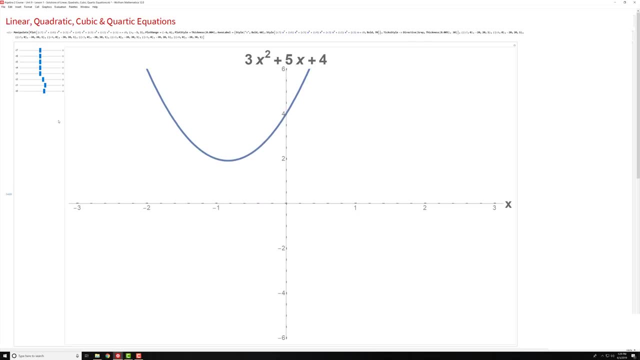 side like this: then I have actually no real roots, but I still have two roots. in total, I have two real roots. So I can see that I have two real roots. So I can see that I have two real roots. I have two complex roots And we're going to learn how to calculate the complex roots with. 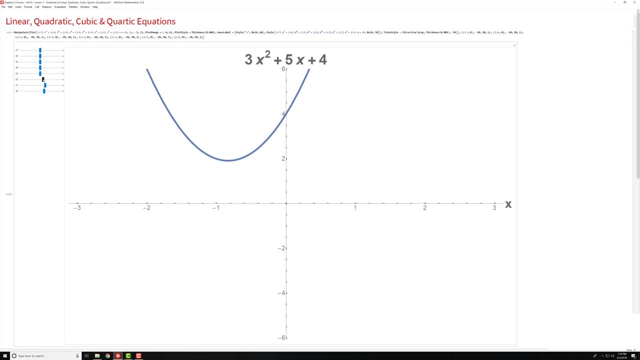 the quadratic formula here very soon, All right. One more thing I'm going to say before I leave quadratics here is: let's do our basic quadratic that's centered on the x-axis right here or centered on the, like this guy, the general quadratic, like 2x squared. or you could say: 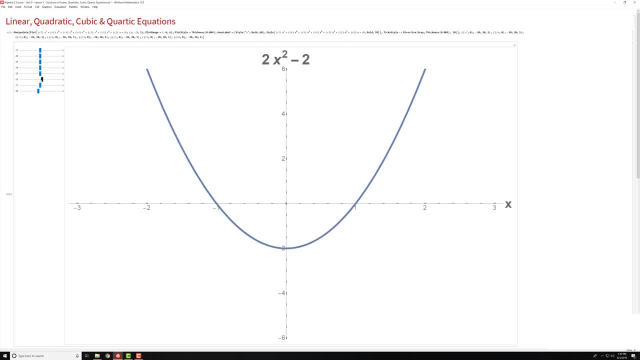 x squared. Notice here that, as I let me make it a simpler one, Let's make it: y is equal to x squared. So here's the general: y is equal to x squared. graph. right, Let me drag it down below And you can see that there's two roots, one here and one here. Now, as I move it up higher, 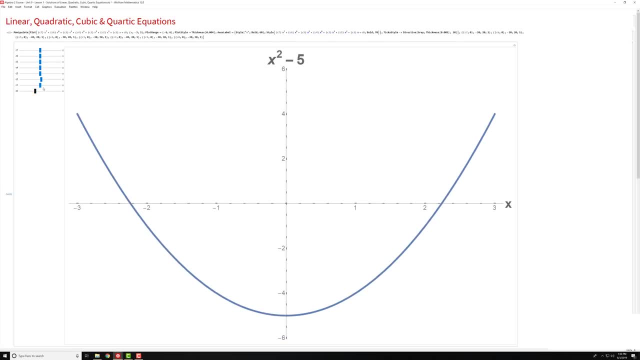 let's go farther down. You see the roots are very far spaced apart because the thing is way below the x-axis. As I make this and shift this graph up, the roots get closer and closer together. You see what's happening. They're getting closer. Here is negative one and positive one, And, as 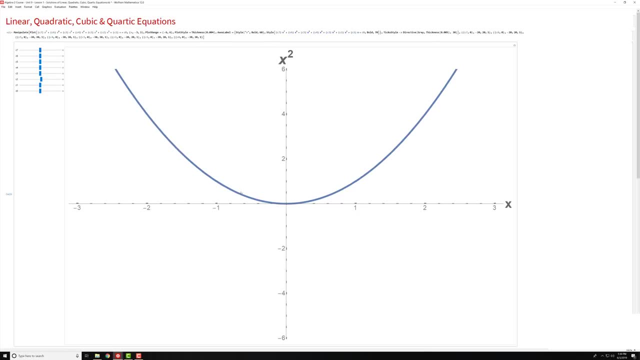 eventually I get to make the graph shift. up to this point, the roots have gotten so close together that they're right on top of each other. The roots were actually right here at x is equal to zero, But there's still two of them. It's a quadratic. There has to be two roots. They're right on top of. 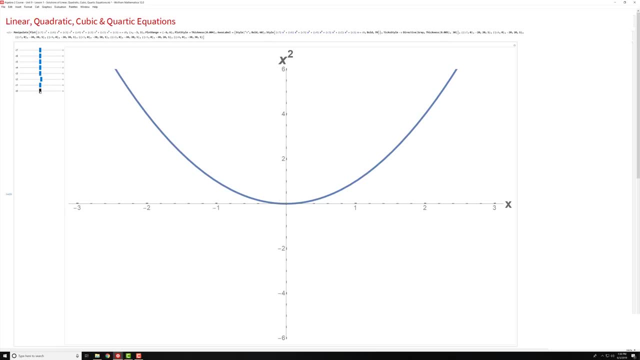 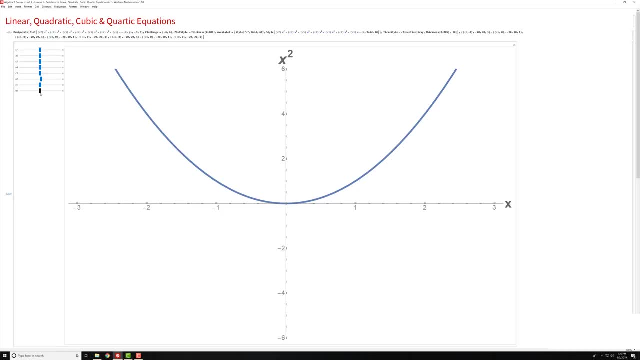 we still have two roots that are right on top of each other. We call that a double root. And then, as we go above the x-axis, we have don't have any real roots at all, no crossing points, but we still have two complex roots, which we'll learn about later. 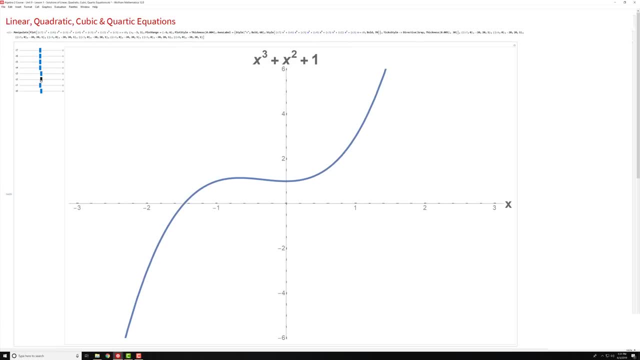 Now let's increase it to a cubic. This is what a general cubic function looks like, And I can play with it to try to make it more like a snake. It's kind of like a snaky function, And so this is what a cubic looks like, And you can see here that the highest power of x is a three. So we 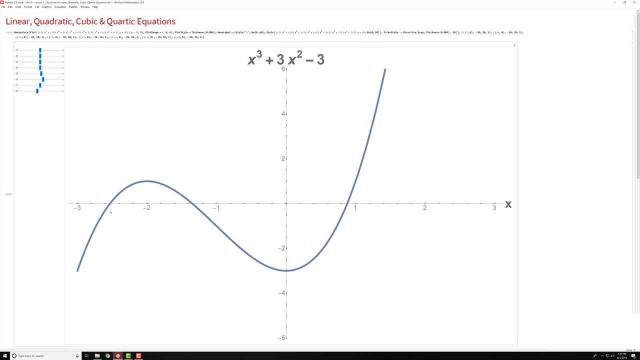 expect three roots of this equation, three crossing points. So here's a crossing point of the x-axis, Here's another crossing point here And here's another one. So there's three roots of this equation. In general, all cubic functions are going to look like this or they'll look like a. 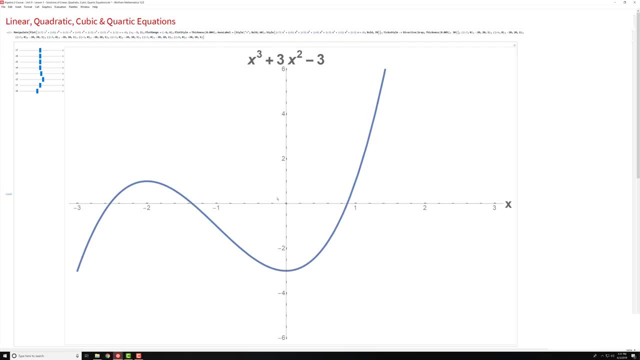 mirror image flipped down below. In other words, it can go up and down or down and up, but it'll still mostly look like a snaky kind of function like this, And as I go and drag this guy down, interestingly, there's only one crossing here of this function. here It still looks like a snake. 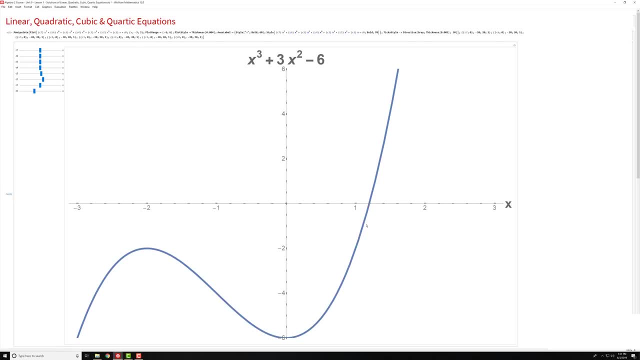 but we only have one root, which means one real root we can see over here. But you have to remember the highest power here is a three. We always have to have three roots total. So here we have one actual crossing point and we have two other roots which you could find. 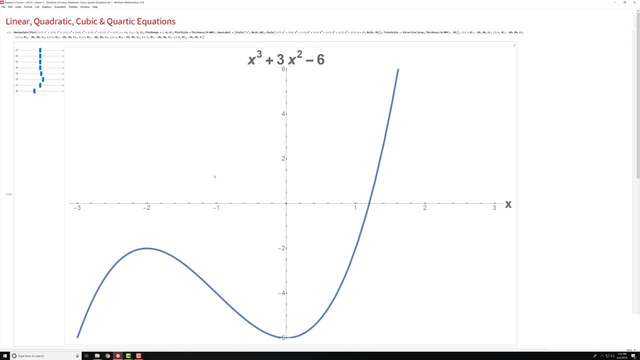 we're going to learn how to solve these cubics later and you'll find out. you'll have two complex roots for a total of three. Two complex roots and then the one real root. here, As I drag the function up, we still have two complex roots and then the one real root over here As I drag. 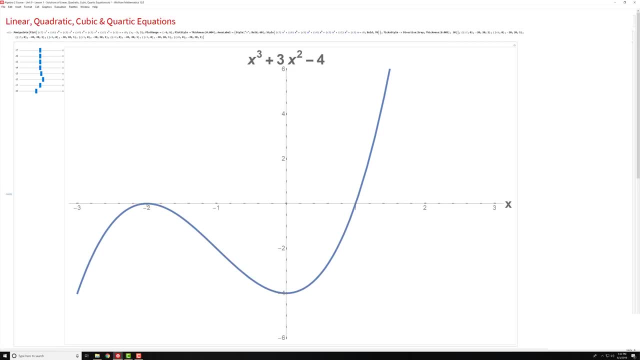 it up here. we have one real root here And notice we have a double root now because the function is now touching the x-axis. And then, as I go through it now we have three real roots: One, here's two and here's three. And as I shift the function up, we still have three real roots. And then, as I go, 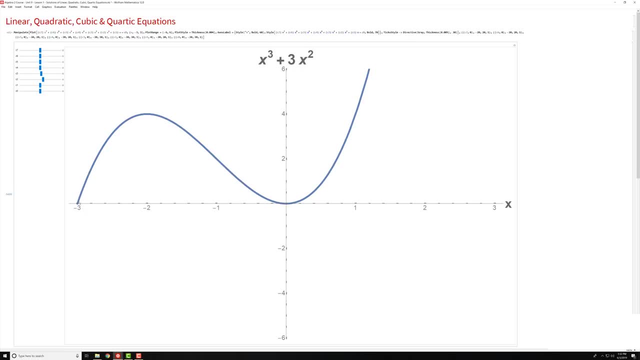 through it. now we have three real roots here, three crossing points, And then we have, on this case, we have the function crossing here. That's a real root. We have a double root now for a total of three roots here, And then as the function gets shifted up, it's a little hard to see because it's 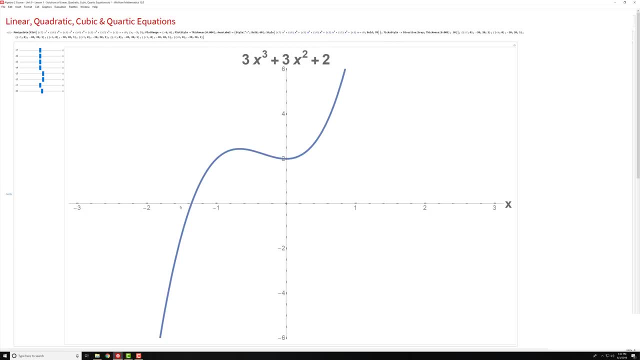 shifted off the screen. That's probably better. We have now a one real root here on the negative side and then we only have. we don't have any other crossing points. So the other two come up to make two more imaginary or complex roots. So the bottom line is: you always have as many roots. 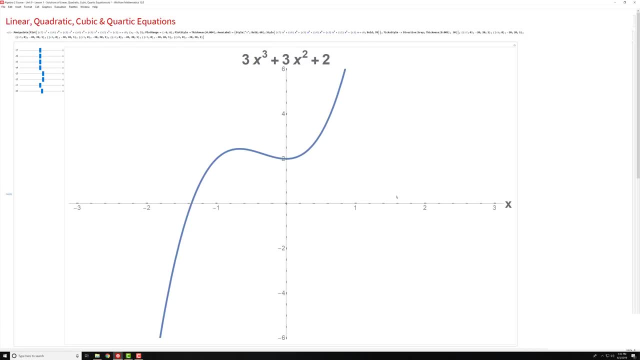 can be complex if you don't have enough crossing points in your graph, And that's what it means to get complex roots. Those are just roots that can't be displayed on a real graph like this, But the real crossing points will show up as roots as well. Now, real quickly, we're not going to go through. 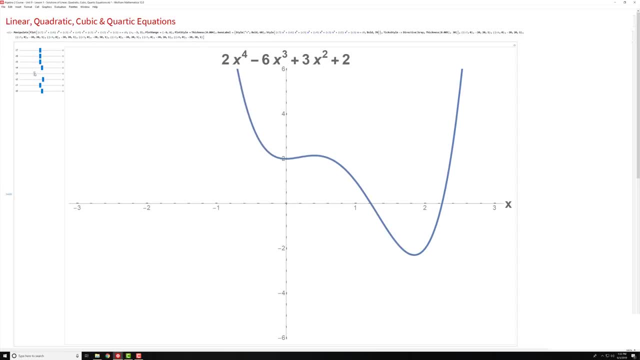 the quartic and higher too much. but let me just show you generally what in general quartic function looks like. You can play around with it, make it look various ways. So here in general you can see it looks like a W. So whereas the cubics look like a snake, the quartics look like a W. Of course, 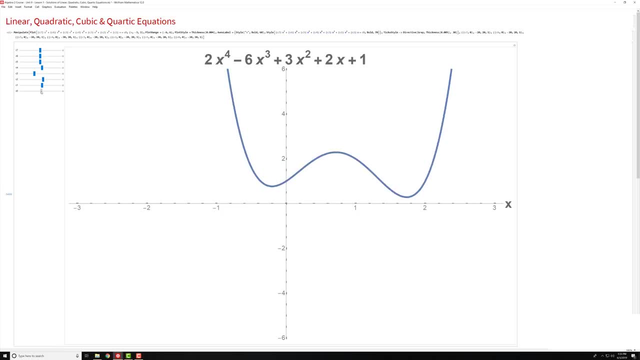 it could be flipped upside down to look like an M as well. But if I drag this function down here, then this quartic equation, this one here that we have printed at the top, has two real roots, because we have two crossing points, but we don't have any more actual crossing points. So the other 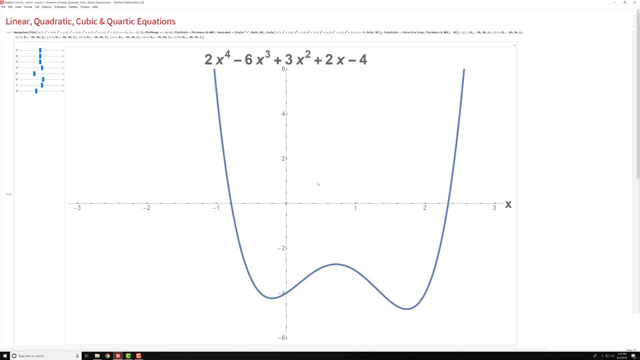 two roots that we expect must be complex. So this graph would have two real roots and two complex roots that you can't see on this graph As I shift it up. it's the same deal. We have two real roots and two complex. Here we have two real and two complex, But now you see that we have two real. 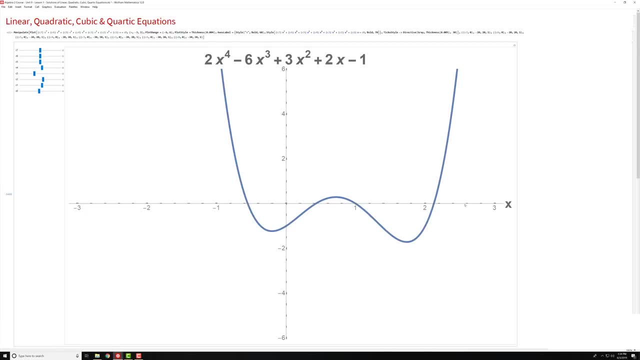 roots and you see, the graph crosses in four locations: One, two, three and four. So this graph has actually four real roots and it doesn't have any complex roots. And as I shift it up, we have whoops. 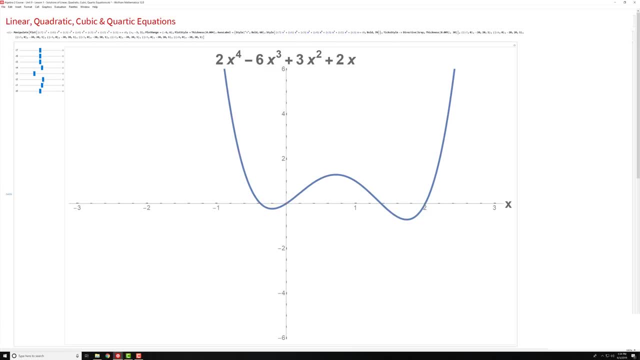 let's go here. We have the same deal here: One, two, three, four real roots and no complex roots. And as we shift let me see if I can get it here And again I'll have the granularity. But as we go, 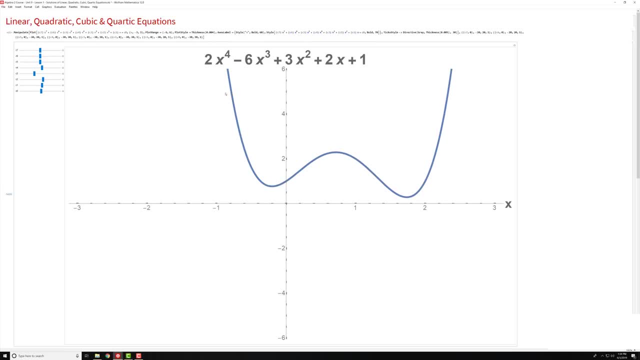 up higher above the axis. this graph, this equation, doesn't have any crossing points at all. So all of this is complex. So you can kind of predict from the graph how many real and how many complex roots you're going to have. Now I'm just going to fly through the rest of them, Because after you, 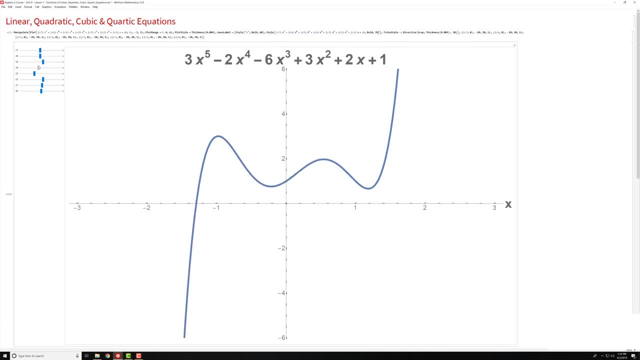 get to the cortex. the rest of them are just kind of hard to kind of visualize. But you can see a fifth order equation still kind of looks like a snaky function And if you push it down like here, you can see you have now five crossing points: One, two, three, four and then five matching. 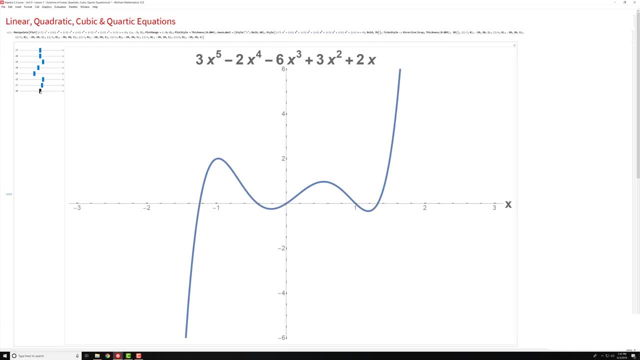 the five roots that we expect. Here are the five real crossing points. If I shift this equation up, changing it slightly like this: now the roots will be one real root and all four of the remaining to equal five must be complex roots, And I can do the same thing by dragging it down here. 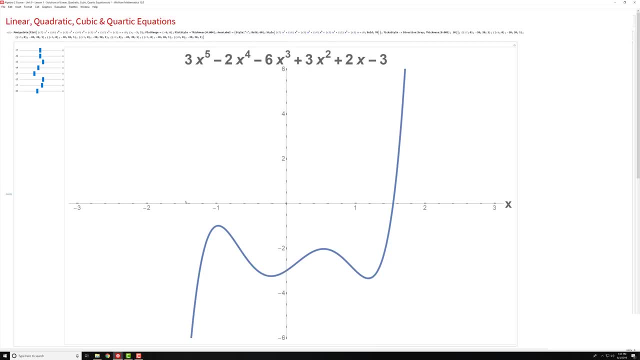 This equation has one real route way over here. and then all of the other four must be complex roots. And then in the middle, as I shifted up and down here, you can see you can have various combinations. here I have the four, the five crossing points in total And just playing around. 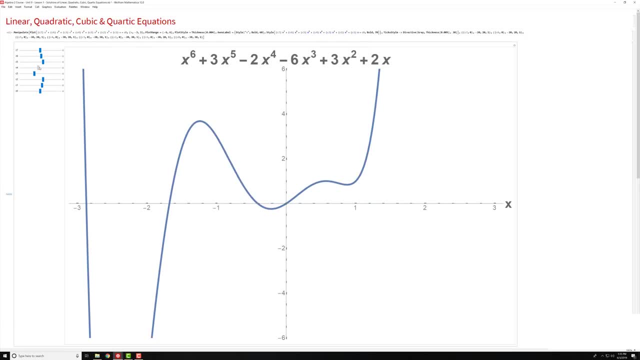 with it more you can. you can make crazier, higher order things like this. Let me see if I can find something interesting Here. you have one crossing point, two crossing points, three, four. So I only have four crossing points that I can see in this function, But we know that there must be six roots because it's 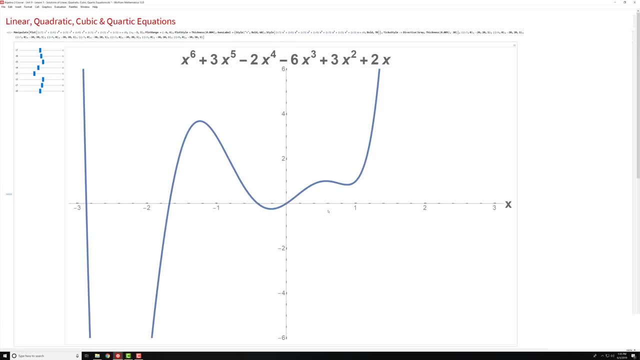 a sixth order, polynomial. So we have four real. therefore we must have two complex. So if you solve and find all of the roots of this equation, then you'll find four crossing points, four real roots, and then the other two must be complex, And then we'll just do one more, just because I know. 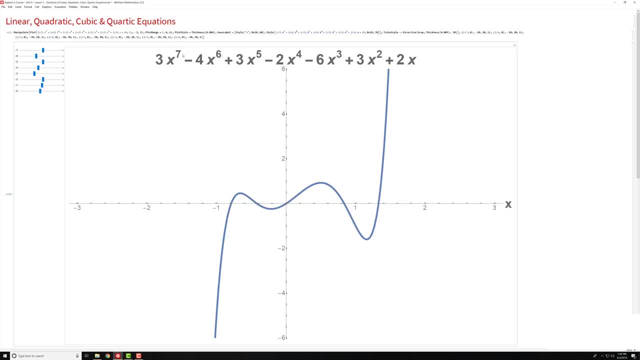 you're curious. The seventh order. see if I can make it look interesting. So this is a seventh order polynomial. You can see the graph of it, But how many crossing points do we have? One, two, three, four, five, we. 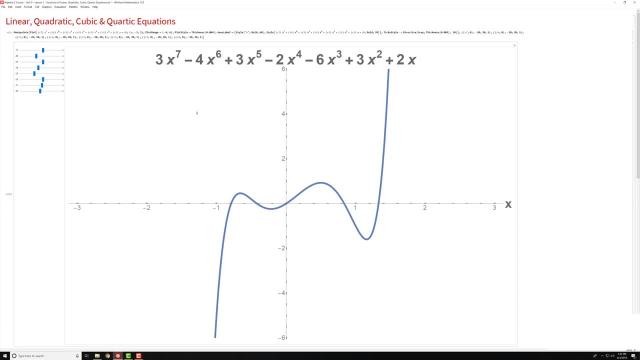 have five real roots. therefore the other two- to make seven- must be complex roots. So I wanted to show you the general idea of what we were doing so that you can get an idea of what real, what, what real roots are and what complex roots really represent. But what I want to do here to close is 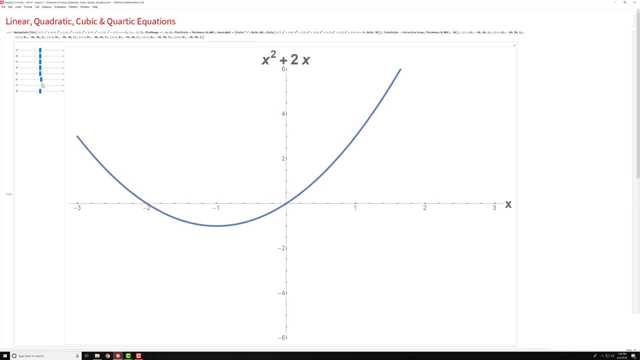 go back to the original thing. When we have our general general quadratic equation, our famous f of x is equal to x squared right And it has two crossing points. That's two real roots. If you have no crossing points at all, that's. 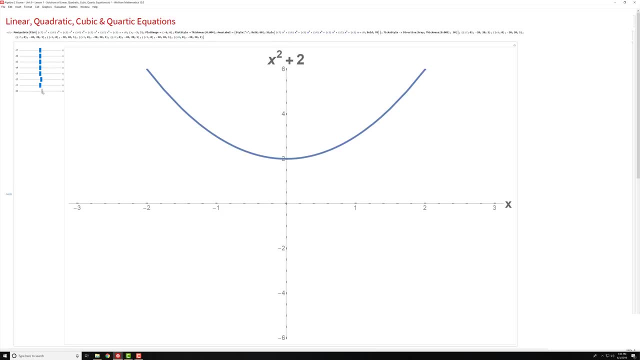 two purely complex or imaginary roots that you're going to get it when you solve this guy. And then, right when it kisses the axis, you have two real roots, which we call a double root. you can see them getting closer and closer and closer together. until now they're just basically right on top of 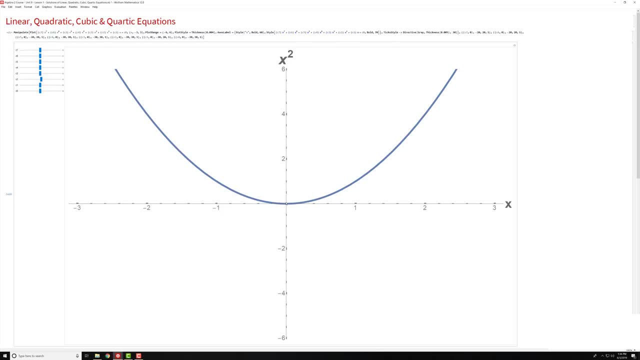 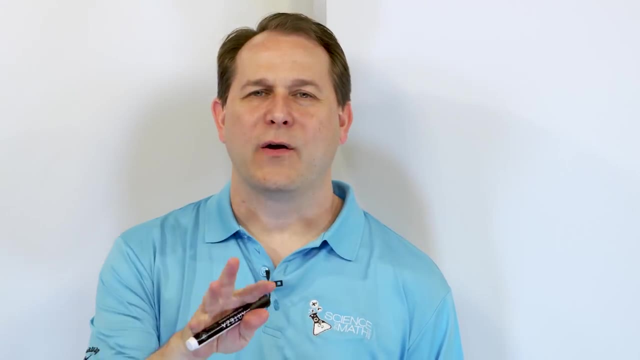 each other, If I can adjust it here right here, at x is equal to zero. So now let's go back to the board and wrap it up with writing down some equations. All right, so now that we've seen the demo of how these roots really behave when we have higher and higher order polynomials, what we 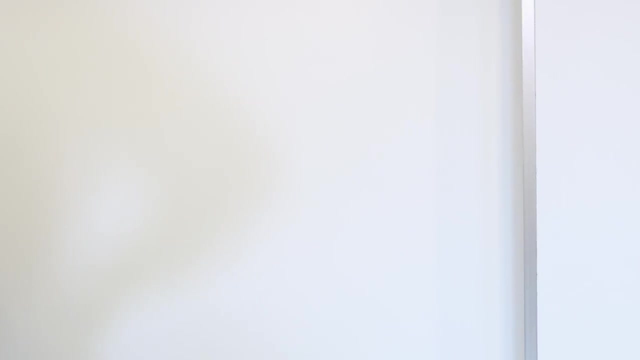 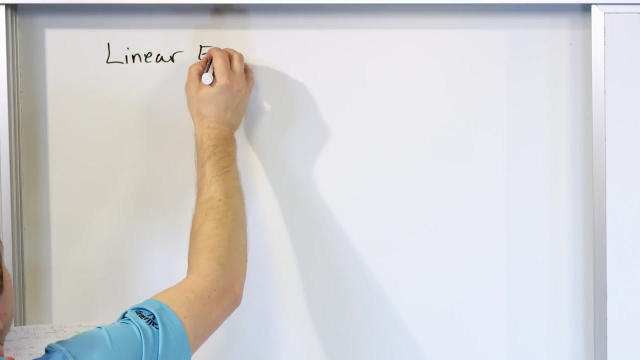 want to do is kind of write some of the things down to make sure you understand and have it all in one place. So the simplest kind of equation that we really have and learn about is called the linear equation. That means it's an equation of a line, And we talked about that many, many 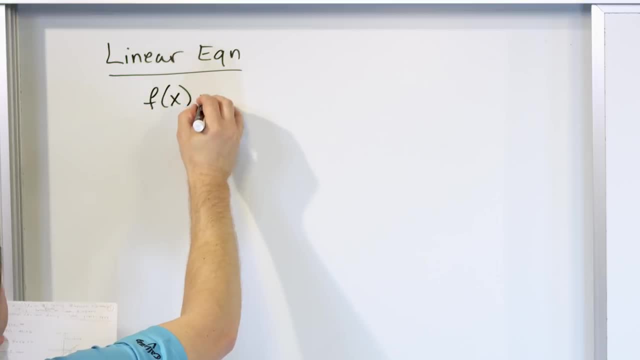 for many hours long time ago, And the equation of a line looks like this: f of x is equal to a x plus b. Now a and b can be numbers, any number, So it could be two x plus three, three x minus four. 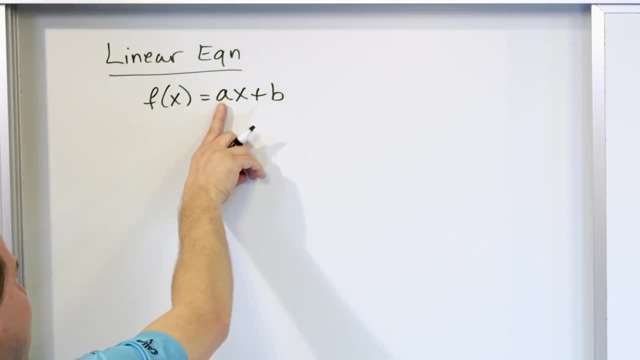 five, you know, and so on, And you can think of this as the slope. whatever this is is a slope in front of this And this is the y intercept, And the way that we find the roots of this guy is we. 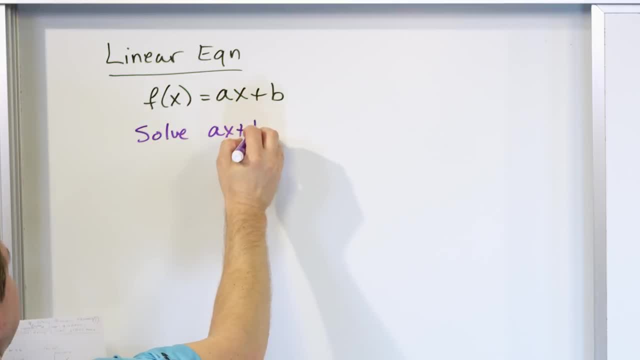 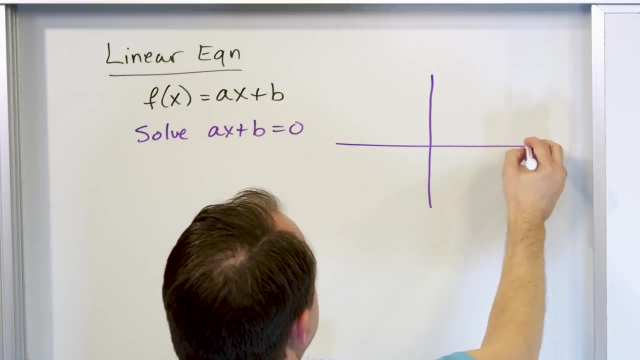 solve the equation ax plus b, whatever it is, equals zero. we know how to solve for x. we move b over, we divide by a, But in general what we get is- we saw kind of in the video there in general 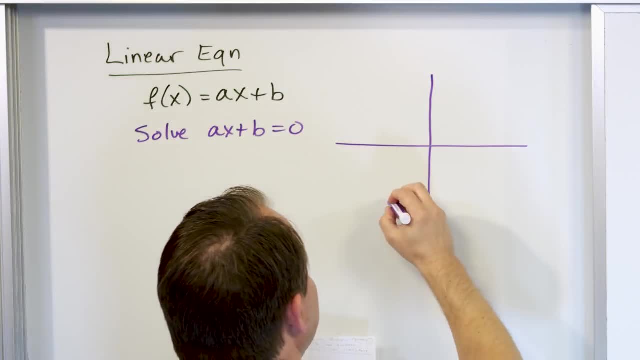 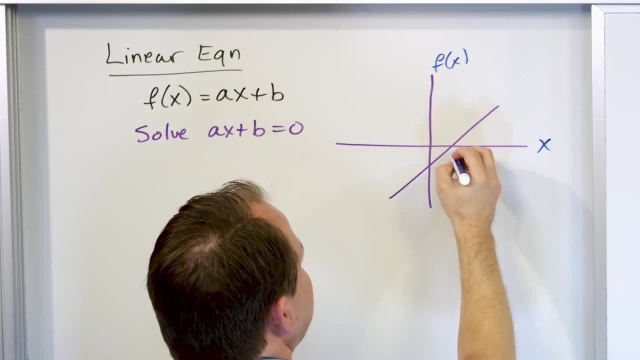 the line could be horizontal with no crossing points, That's true, But in general it's going to have one crossing point. In this particular case, this is x plus b and we're going to have x. this is f of x. The crossing point is actually right here, at this value of x, right here. So this: 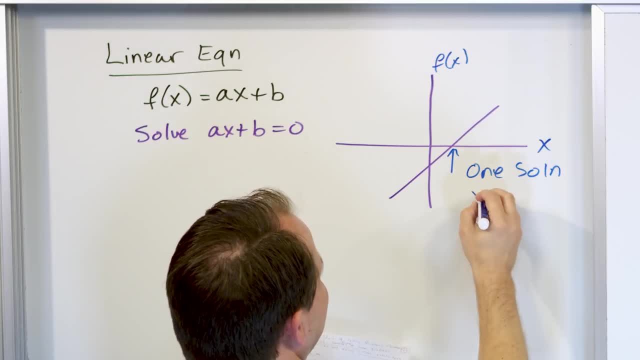 is one solution, And you could say it's like an x is equal to two or something. In fact, I'm just making this up, I'm just, you know, giving you an example. As we saw in the video there, there's one. 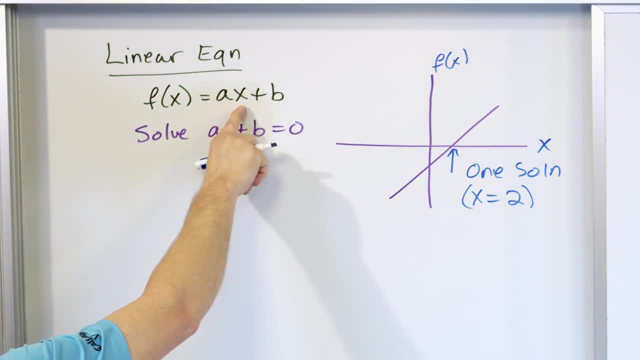 crossing point. There's one solution, because we expect one solution, because the highest power of x is just equal to a one. Now, moving up the complexity a little bit, we have the famous quadratics, quadratic equations, Which we're going to be using and zooming in on almost entirely in this lesson. But the quadratic 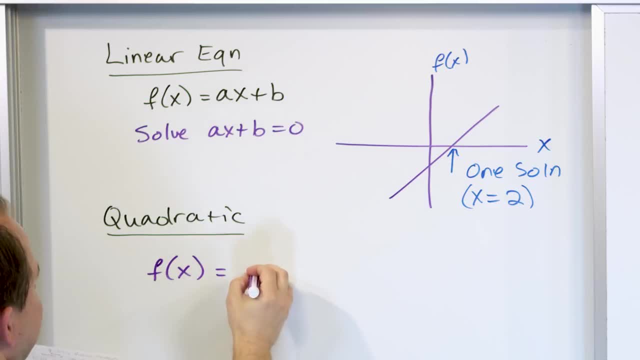 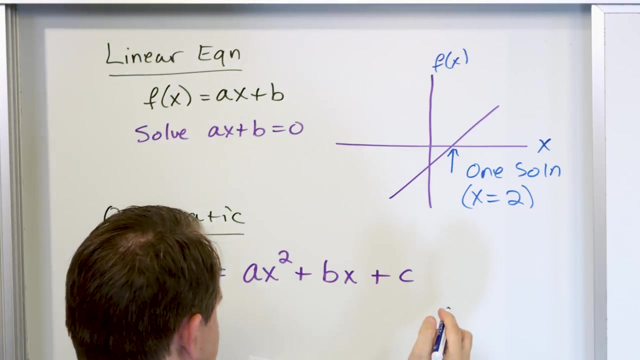 equations in general look like this: All of the quadratic equations have the form ax, with a power of two plus some number, times x plus some other number. Now a, b and c can be any value, except for one exception, and that is that the power, the value here a, cannot be equal to zero. In other, 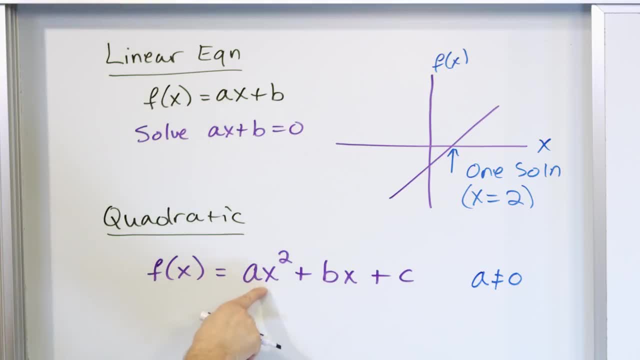 words. for it to be a quadratic, you have to have some. you can't have zero here, Otherwise it would kill the quadratic term entirely, right? So in order to find the roots of the quadratic equation, how many crossing points? 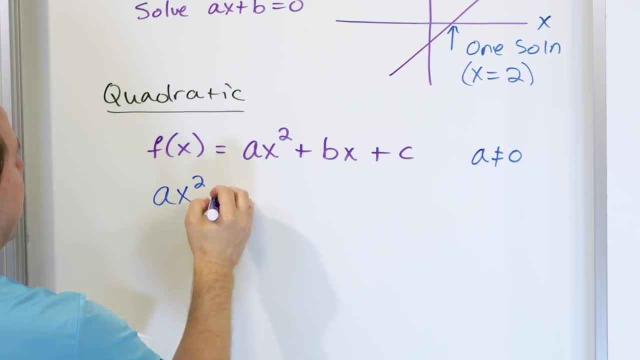 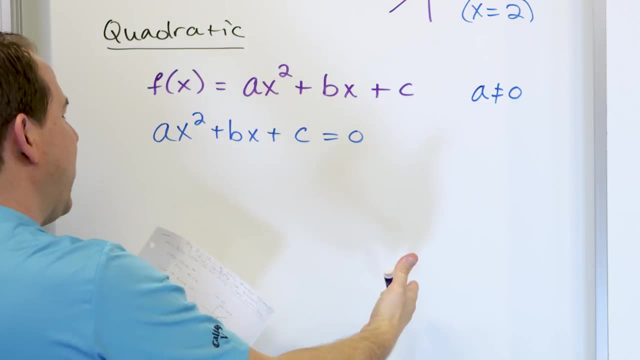 you have. what you do is you take this quadratic equation- you have ax squared plus bx plus c, and you set it equal to zero. Then you factor it, or you could do completing the square, like we've been doing. We're also going to learn about the, or we will be doing actually completing the square to. 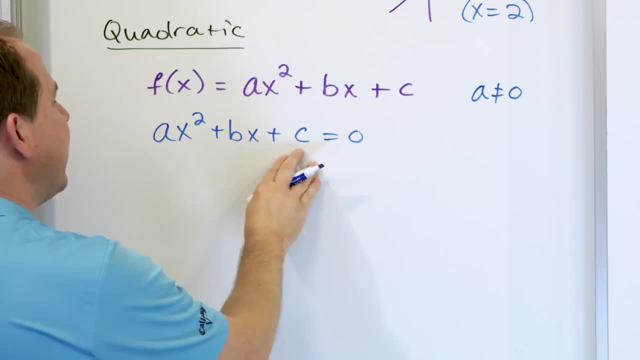 solve this guy. We'll also be using the quadratic formula to find out the values of x that satisfy this equation, And then the main idea is: what is the solution? And then the main idea is: what is the solution? And then the main idea is: what is the solution, And then we have to figure out the 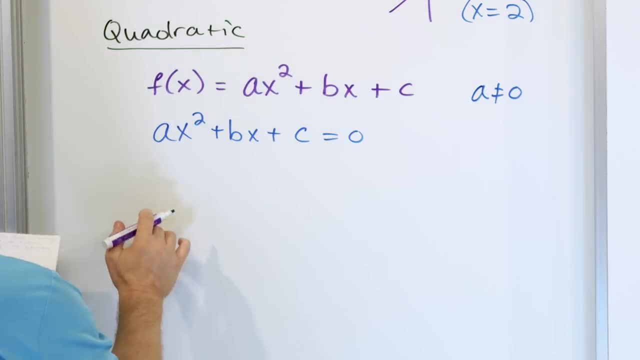 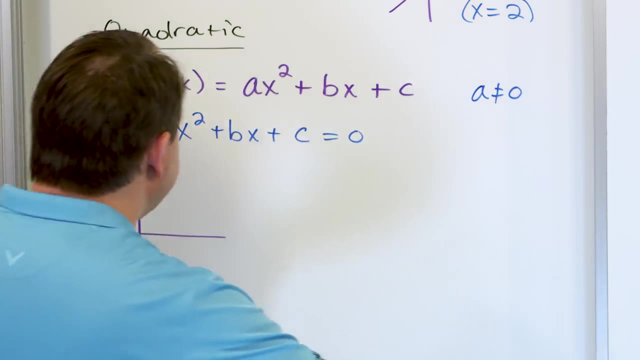 what does the values of that equation actually represent? Well, there's a couple of different cases and we saw some of them in the video there, in the demo there, But let me just draw a couple of cases here. If you're quadratic, depending on the values of a and b and c. 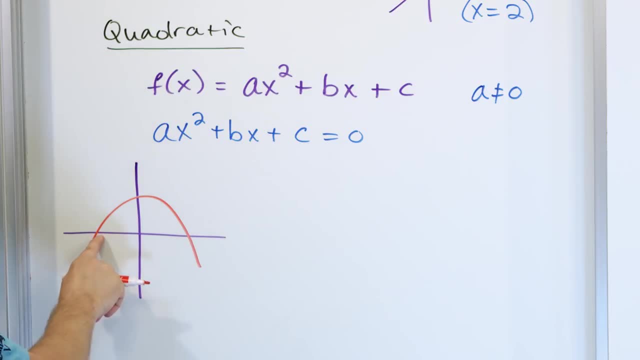 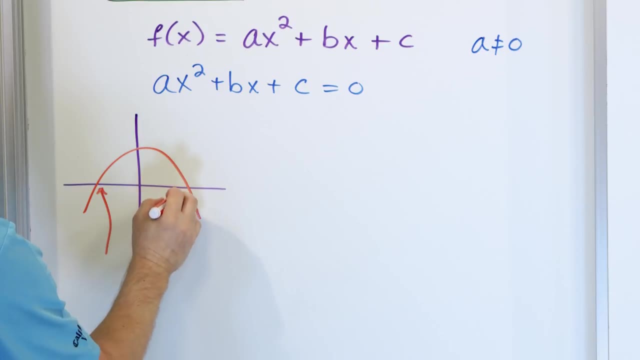 happens to look something like this: an upside-down parabola. then there's two crossing points, because you're setting the value of this equation equal to zero. So this is going to be a solution, and this is going to be a solution. 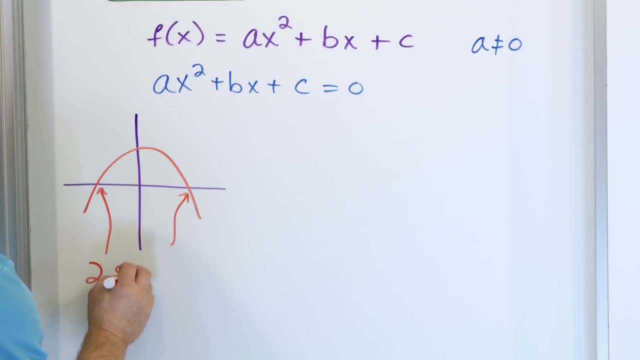 There's going to be two solutions, right. So you're going to have two solutions right. And just to kind of make things up, you could say that x would be negative, 3, and x could be positive, you know, 2 or something. 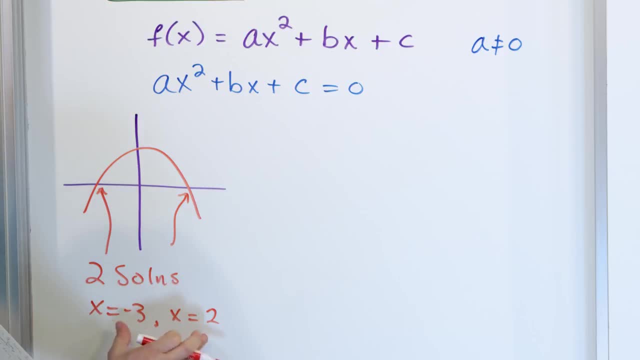 I haven't exactly drawn it, But you see the idea. You have a positive, some two positive-negative value. in this case, You have two actual roots. What are some other cases that you can get with quadratics? What does it actually mean? right, 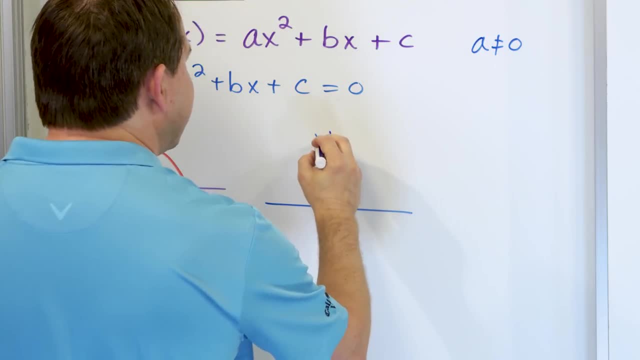 Well, you could have a case like this. You could have, of course, a parabola that dips below the x-axis, like this. So you have two crossing points still. You have a crossing point here and a crossing point here. 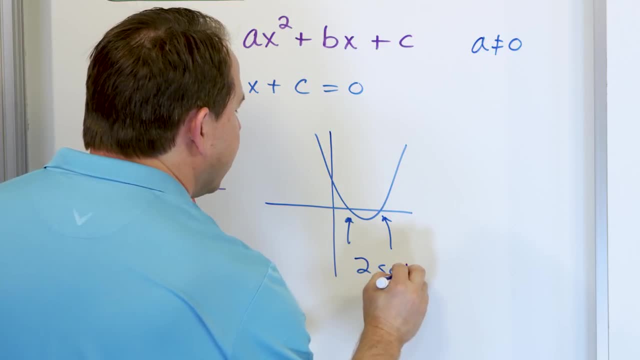 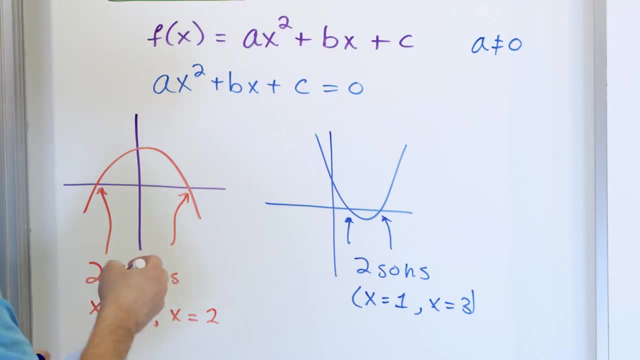 You still have two solutions. You have two solutions And the values of these solutions are both positive. So it might be, for instance, x is equal to 1 and x is equal to 3.. Those are two real solutions, But there are other ideas and other kind of possibilities, right? 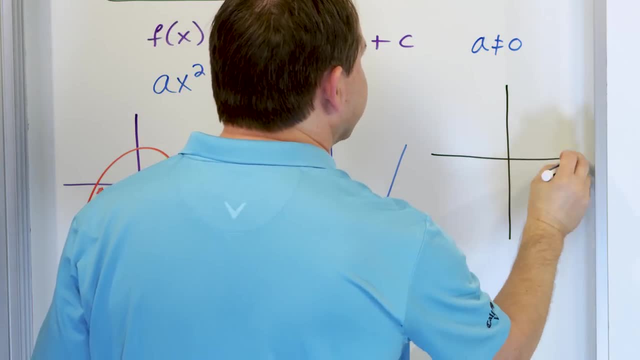 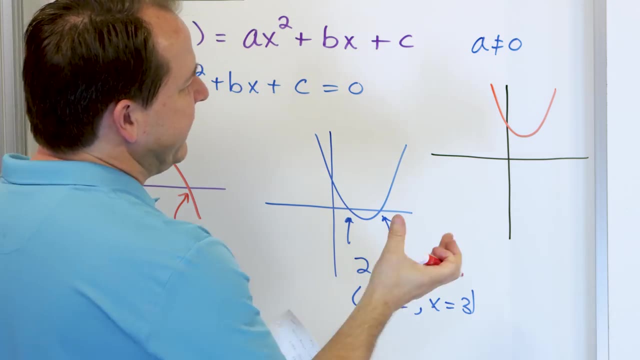 You could have. let's go over here and draw a couple of different possibilities. What if you had the parabola, as we saw in the demo there, floating kind of up above the x-axis? Well, you see, there's no crossing point. 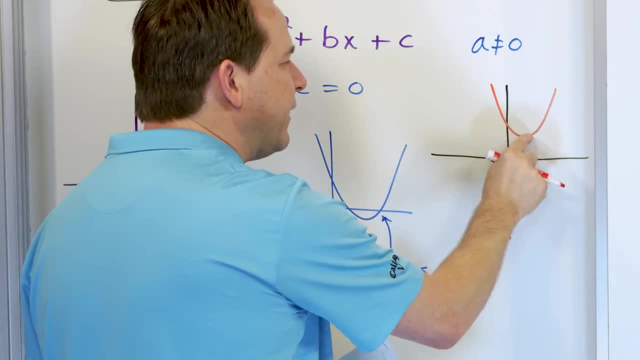 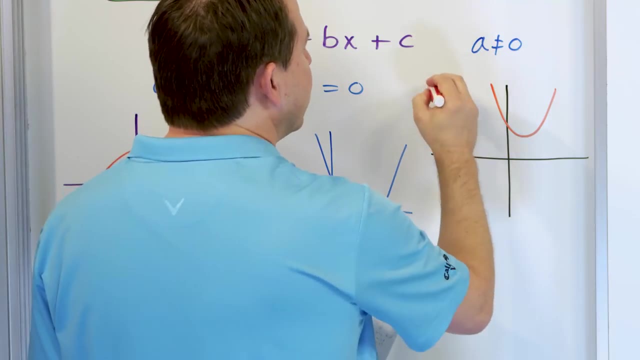 There's no values where this equation actually equals 0. All of the values of the function are all above 0. So there are no crossing points. So there are no real roots, right, So no real roots. But what we're going to find is there's still two roots of the equation. 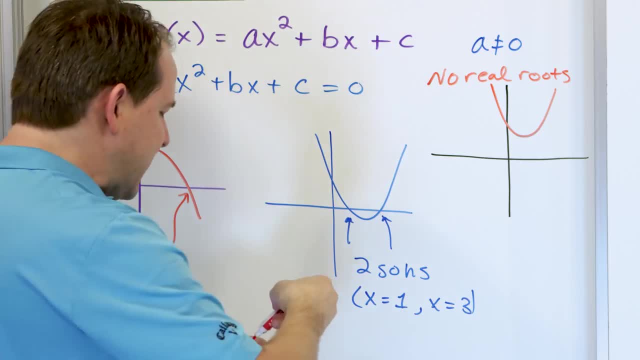 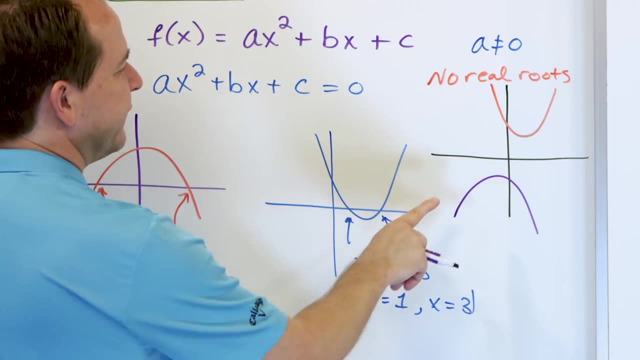 They're just both complex, which involve imaginary numbers. Now another example of when you would have no real roots is what if the equation kind of is down below but going upside down, So you see all of the values are negative for this function. 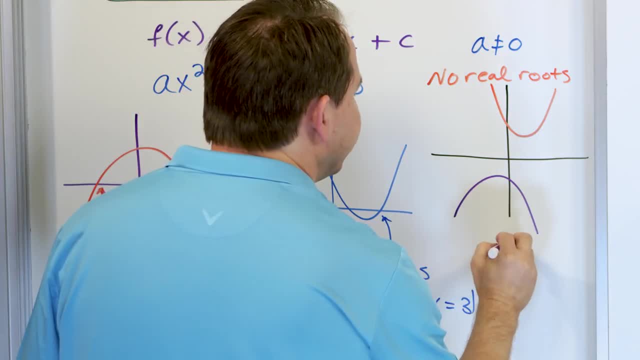 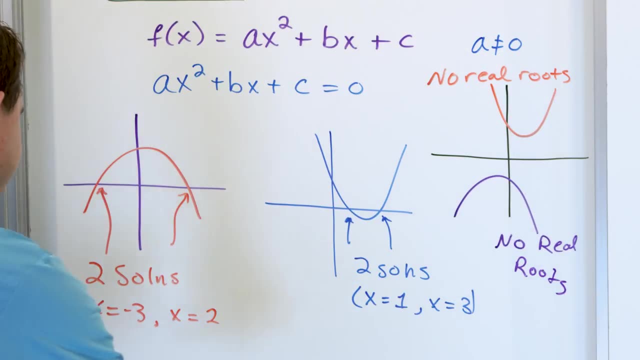 They do. They do not ever cross the x-axis. So, again, there's no real roots here either. No real roots, right? And then, of course, we have the one final example that we really need to talk about, which is the case that we kind of illustrated in the video here. 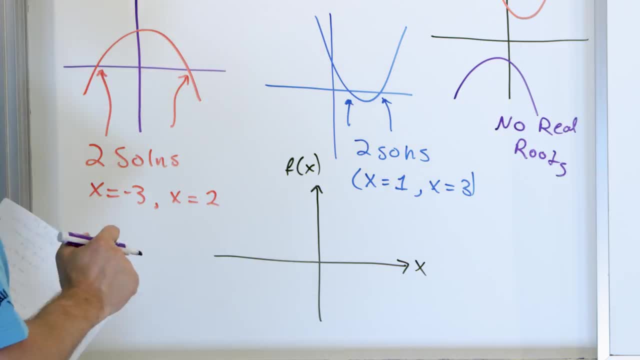 in the demo here just a minute ago, And that is the case of the double roots, right. So what if you have the quadratic come down and just barely touch the axis, but only in one spot? It can be at a positive-oriented curve, like there. 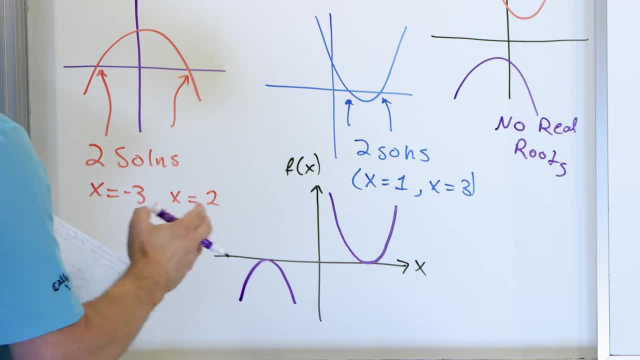 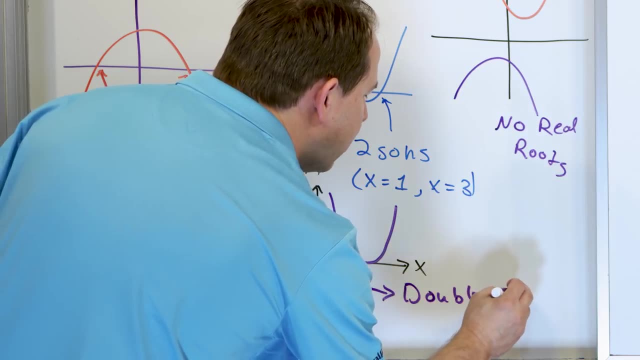 or it could be in a negatively-oriented curve where it only touches in one spot here. In either case, there's still what we call two roots, but we call it a double root, And when I was learning this stuff the first time, the idea of a double root really confused me. 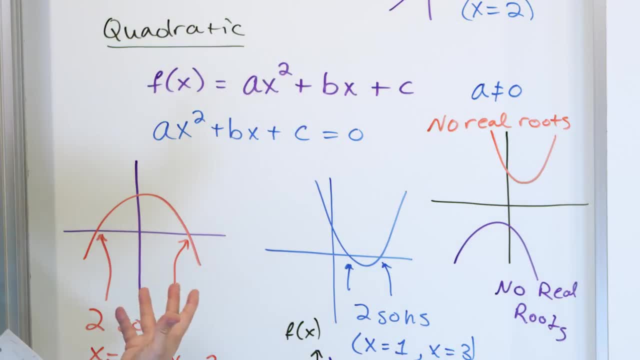 Why is it a double root? Well, it's because, as I showed in the demo there, as your quadratic goes closer and closer and closer to the axis, the roots get closer and closer together. Eventually, when it's just touching the axis, there's still two roots. 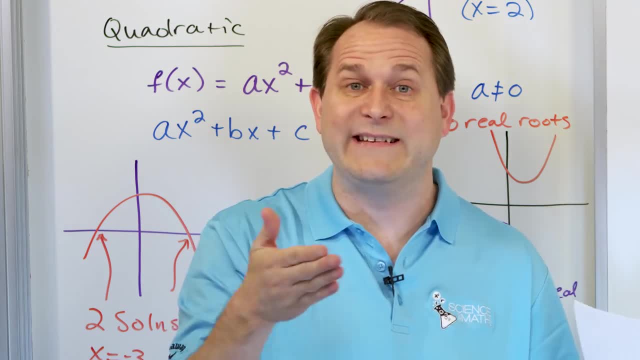 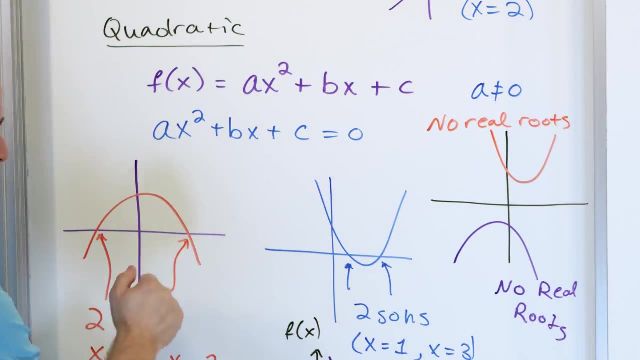 but they're infinitely close together. They're basically on top of each other, so they have the same exact value. X is equal to, you know, 1, and then X is equal to 1.. They count twice. You still have to have two roots. 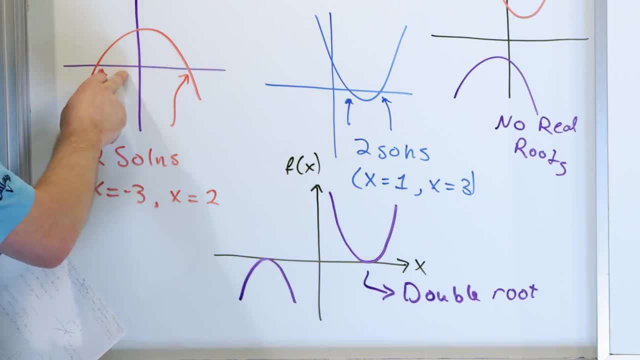 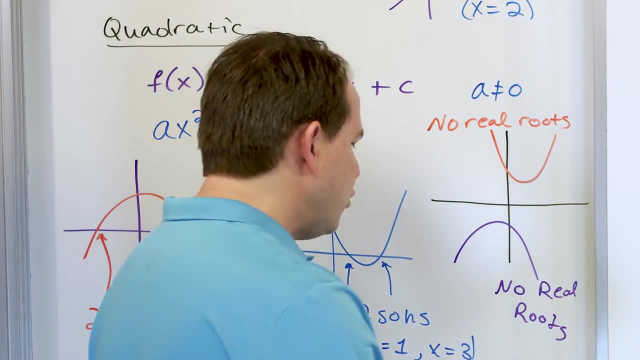 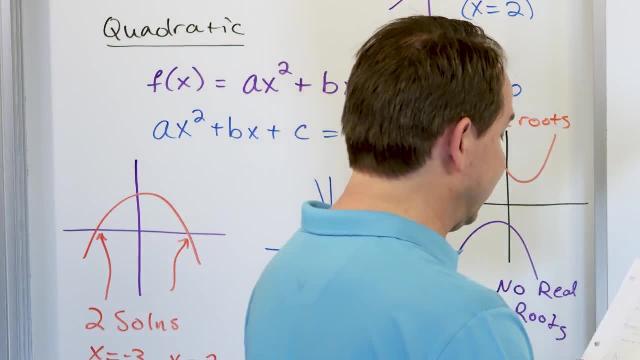 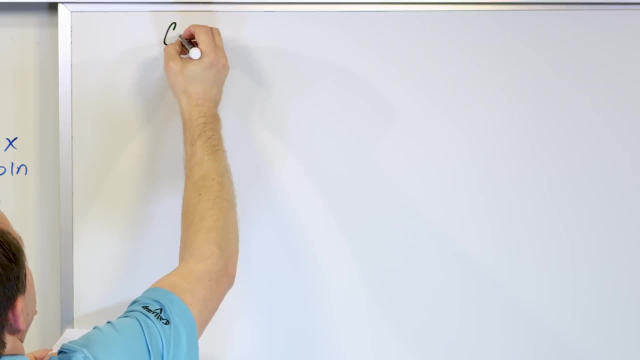 continue learning how to solve these quadratics, which is what we're going to be doing mostly in this section. But this is an overview section and I wanted to show you. I want to talk about more than quadratics. We talked about this in the demo cubic equations. 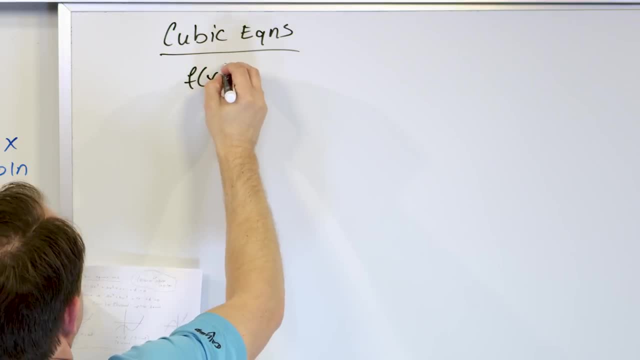 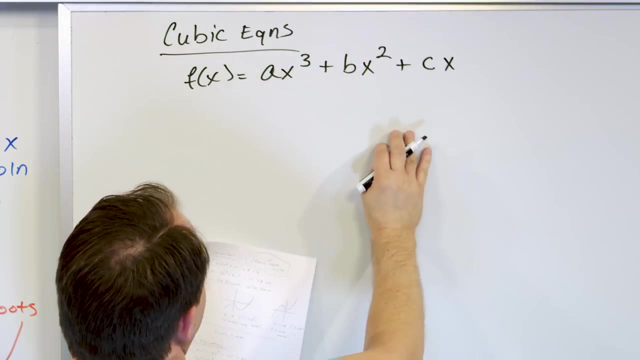 The general form of the cubic equation looks like this: F of X is some number times X to the third power, plus some number X squared, plus some number times X plus some number right, That's F of X. That's a cubic equation. 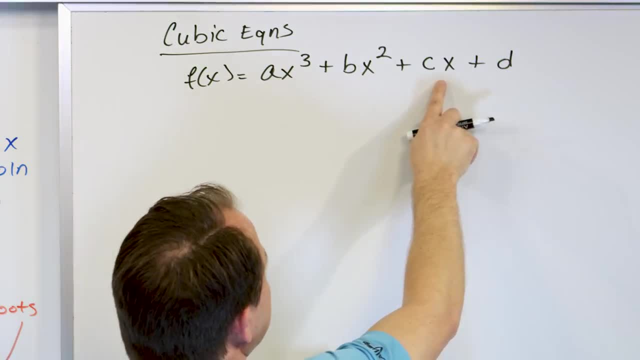 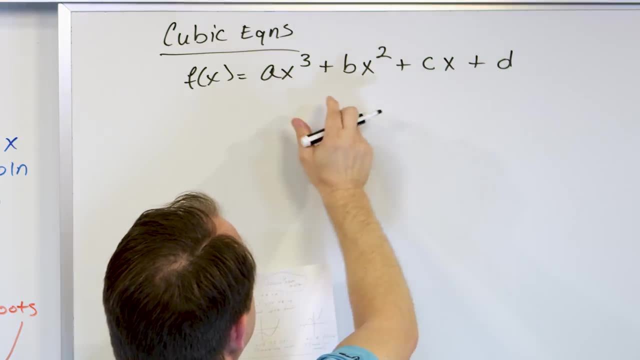 This number here needs to be something other than zero, but any of these other ones can be zero, like B, C or D could be zero. In other words, it doesn't matter what the rest of this thing is. It's a cubic if the highest power is a three. 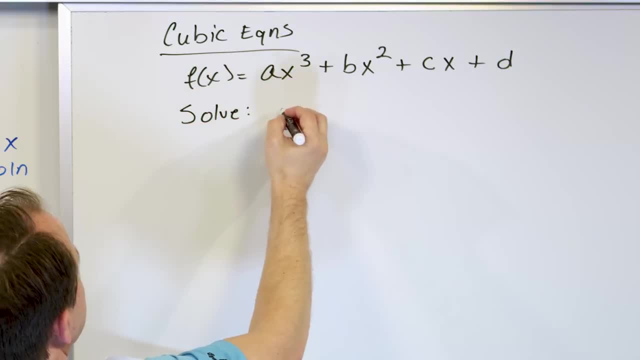 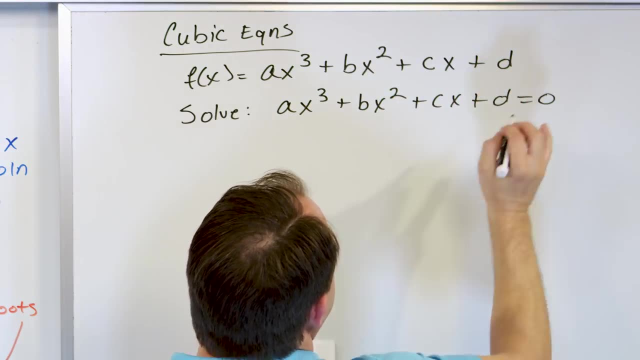 So, to figure out the roots of this guy, what you're going to be doing is you're going to be solving this equation- X to the third plus BX squared, plus CX plus D, And you're going to set that guy equal to zero. 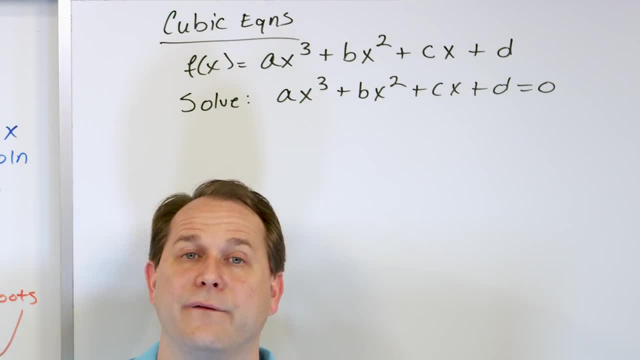 And we're going to learn, as we get a little farther in the algebra, how to solve cubic equations. We're going to learn how to factor things out and how to separate and divide things, And we're going to figure out the roots of this guy. but graphically, what does it actually mean? We saw in the drawing that if we were to divide a cubic equation, that if we were to divide a cubic equation and we're going to learn how to factor things out and how to separate and divide things. 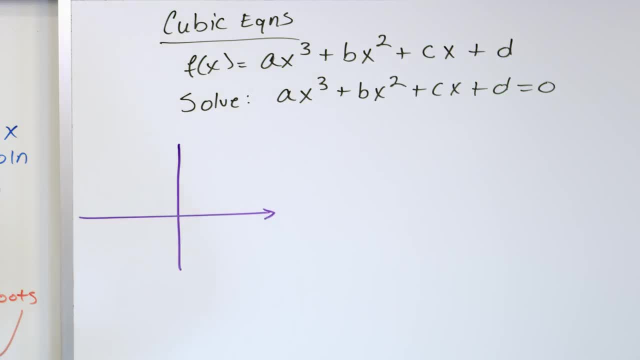 the demo in general what it means. but I want to make sure everybody understands Now in general the cubic equations, I call them these snakey functions. They go up and then down and back up. So you see there's three crossing points corresponding to the three solutions that we expect to find. So for instance, 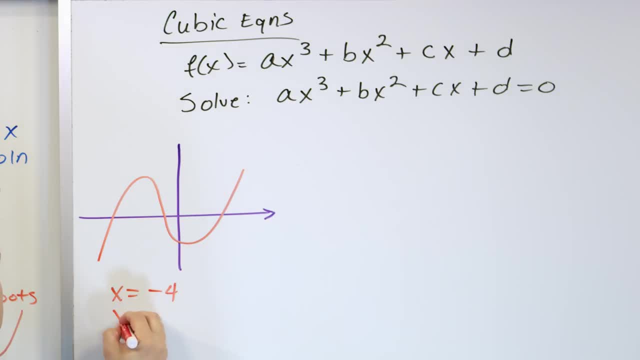 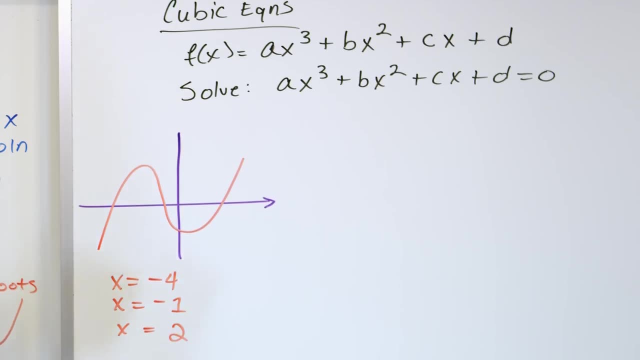 you might say that x is equal to, like over here, negative 4.. You may say that this root is over here at negative 1, and you might say that this root is at positive 2 or something. So there's three real roots here, three real roots. 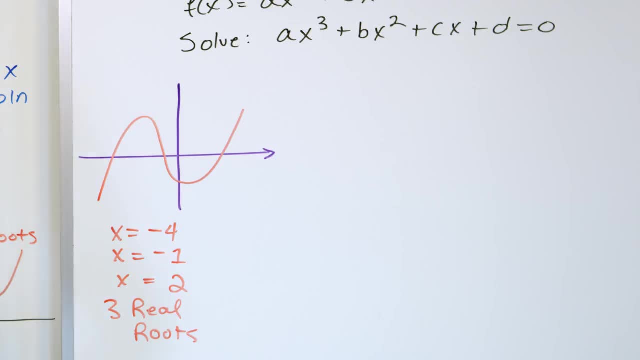 for this equation, if this is what it were to look like. But there are other possibilities which we saw over there when we did the demo there, And there's infinite possibilities really. but you might have one that goes up like this and then snakes down but doesn't quite go below the axis again. So 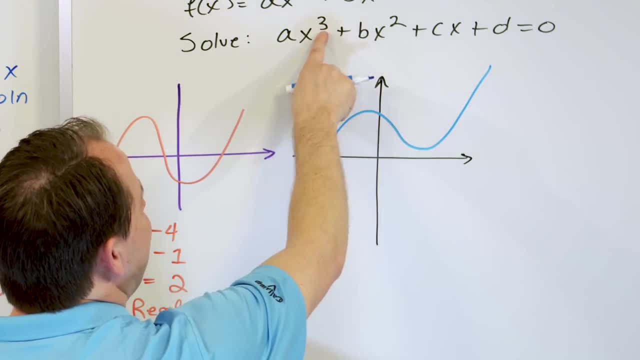 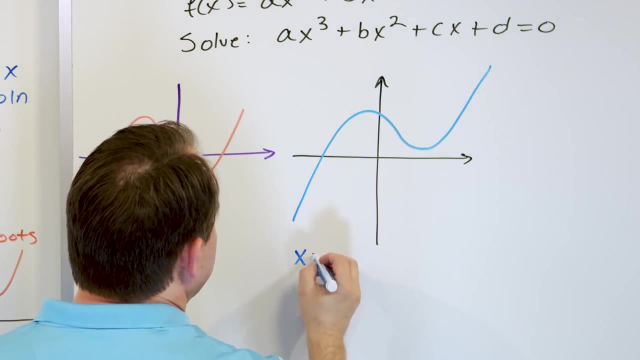 in this case, you have only one real root. The other two, which you have to have to make three, are going to end up being complex roots. So what you might say, for instance, is that your real root is going to be: x is equal to like let's. 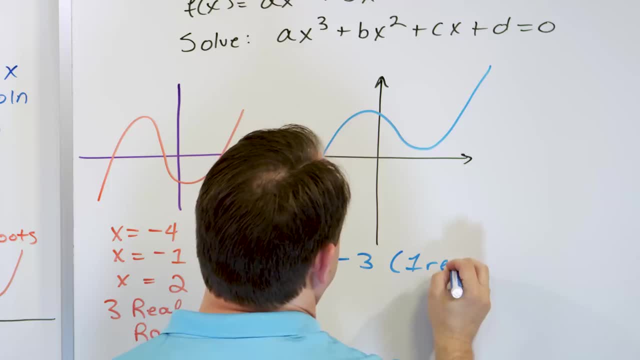 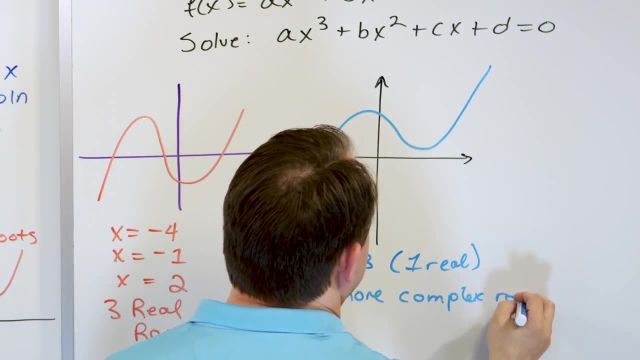 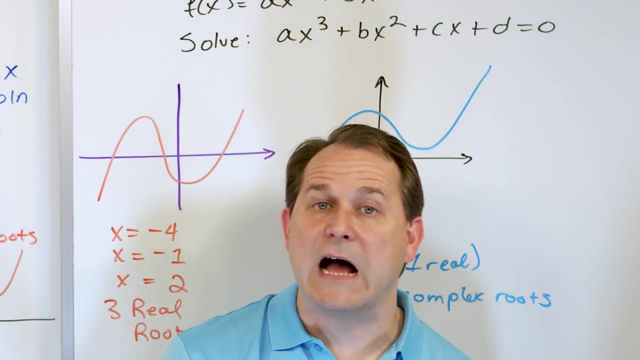 say negative 3,, one real root And then the other two roots, two more complex roots. So in other words, when we learn how to solve these things, we might find out that the real root is negative 3, and the complex roots might be 1 plus i. 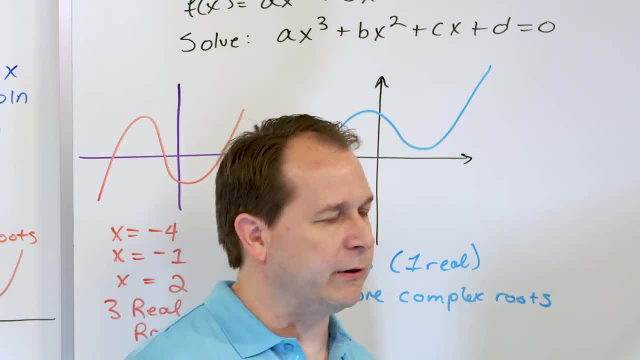 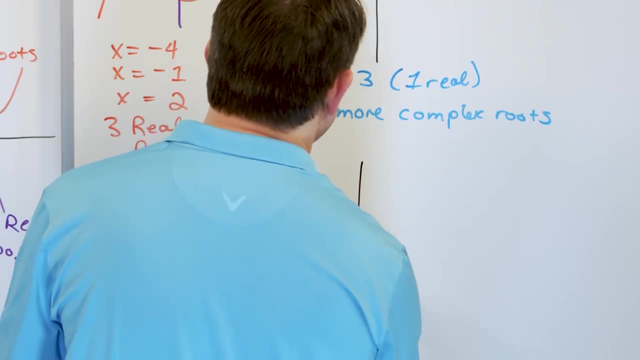 that's a complex number. and then 1 minus i, that's another complex number, for a total of 3.. And then one more quick case: since we're just trying to be, you know, explicit about everything, we might have something that looks like this: We might have the function go back bend. 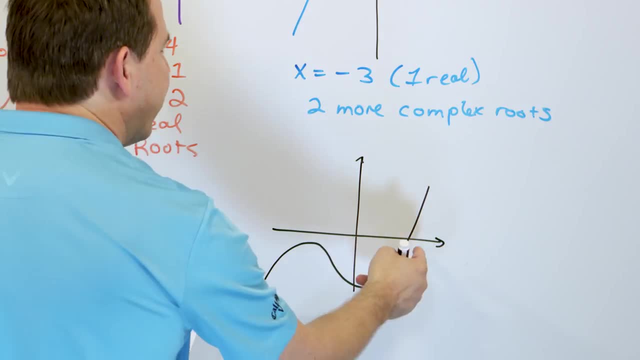 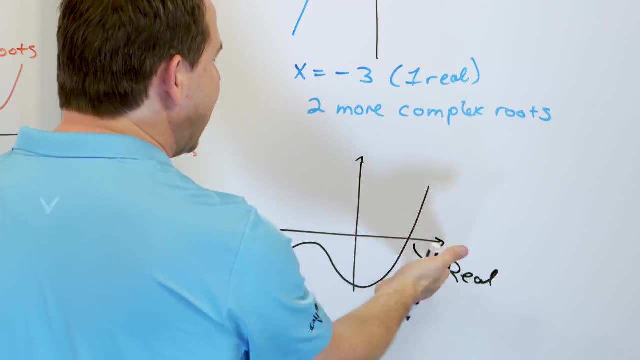 back below and then go up, like this. It's a similar kind of situation: You have one real root here right, and you have two more roots that are complex, which we haven't learned how to solve yet, but they have to add up to equal 3.. 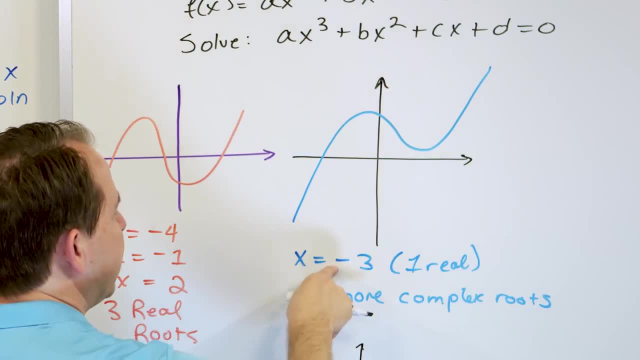 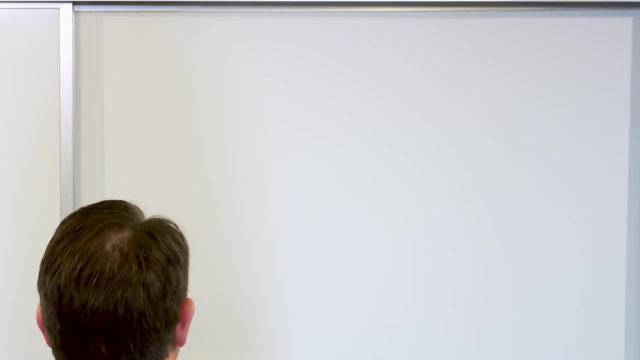 So three real roots, three roots total, only one of which is real. three roots total, only one of which is real. And we're only going to do one more here. we're going to talk a little bit about the quartic equations The way you. 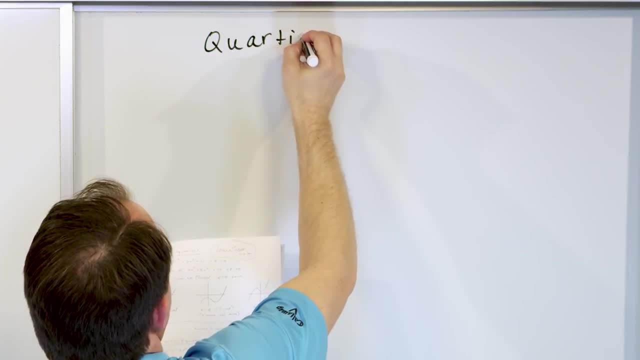 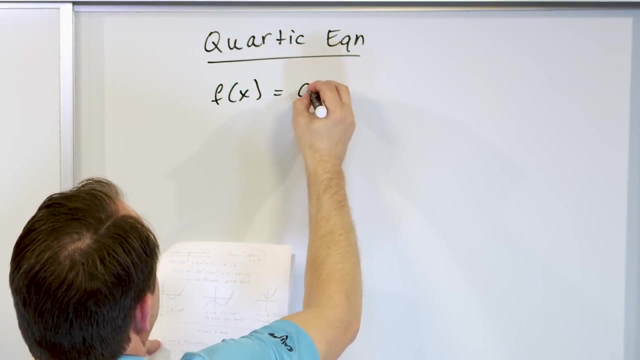 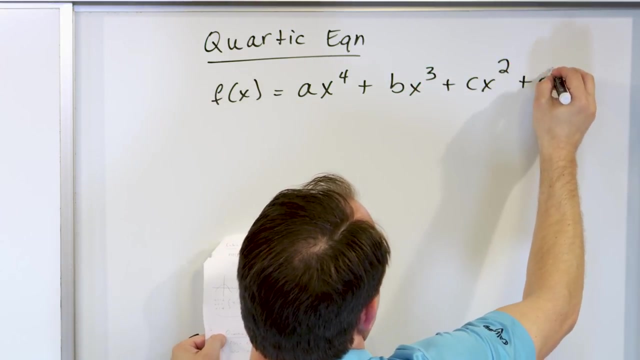 spell. it is like this: quartic equations, right? And so the quartic equation looks like this: It's a fourth power, ax to the fourth, bx to the third, cx, squared dx, e. So I have to use different letters, right? And if you want to solve this quartic, 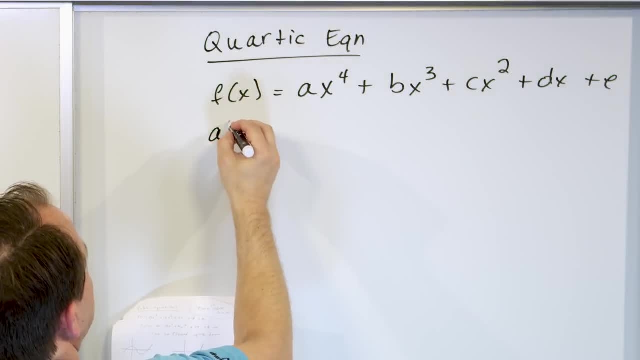 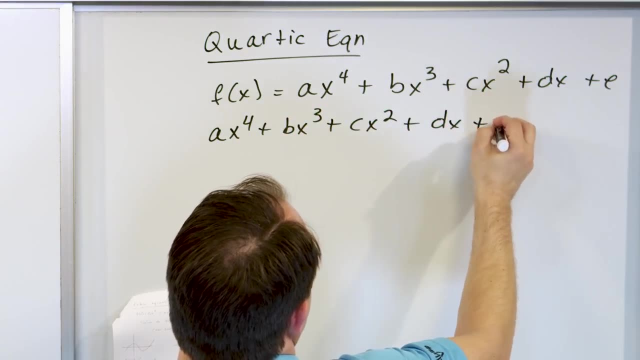 equation to figure out where the roots of it lie. then you just set this whole thing equal to zero to the fourth bx, to the third cx. squared dx plus e equals zero. now we have no idea how to solve this- we haven't learned that yet- but there are methods and techniques you can learn to figure out the. 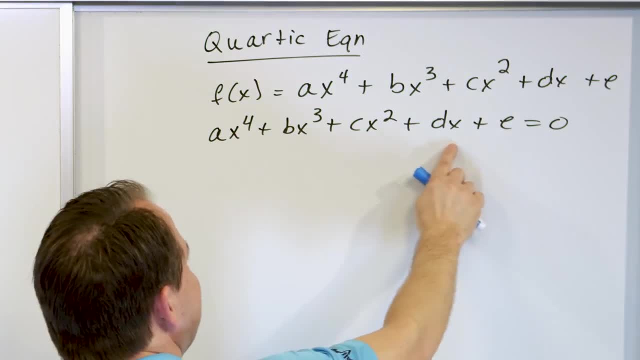 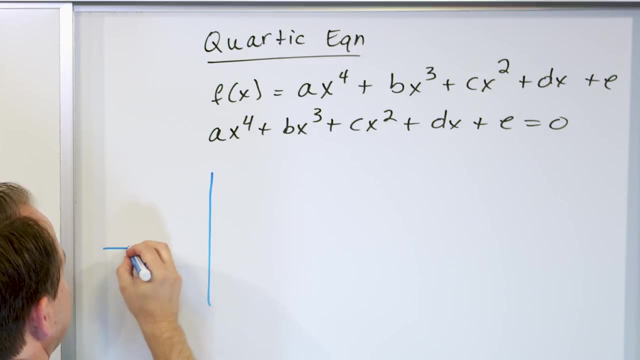 values of x. there's going to be four values of x that are going to make this thing equal zero. four solutions, because it's a fourth power. that's what we expect. so, in general, the quartic which we kind of learned, we looked at in the demo there, in general is going to look like this: it's going: 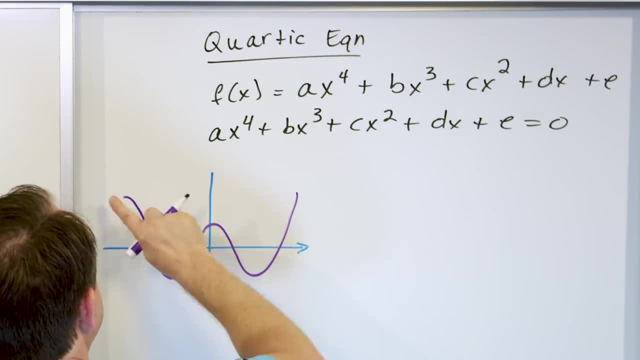 to be a w of some kind. it's going to go down and up, kind of like this right now. of course it can be flipped upside down so it can look like an m, right, but in general it looks like a w. so in this case you have one, two, three, four crossing points, so you have four real solutions like this and: 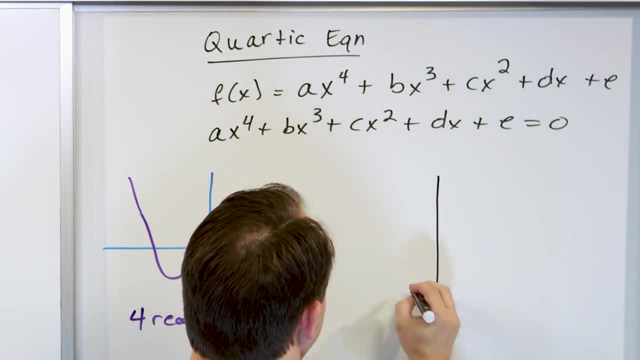 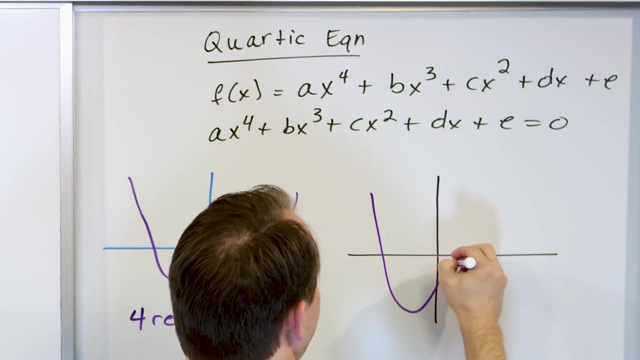 then of course we have other possibilities. let's take a look at some of them really quickly. what if we had the case which we briefly did examine something like this again: it goes down and up, but not quite high enough, and then it goes back up, like this: we have only one. 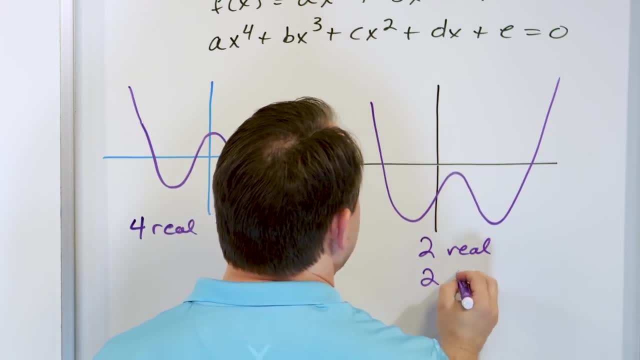 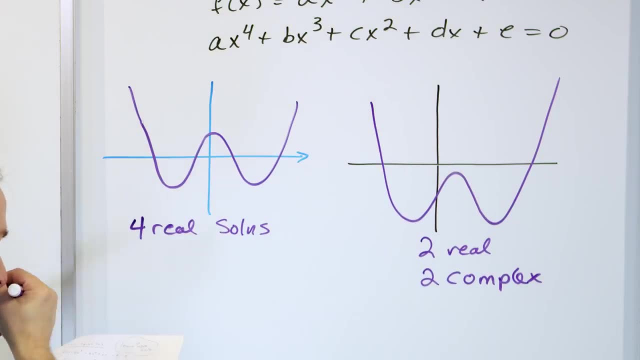 two real solutions and two complex. we can't represent the complex solutions on this graph, but we know they have to exist because we know there has to be four total. and then we have the final case which i want to talk to you about, and then we're basically almost to the end of all this. 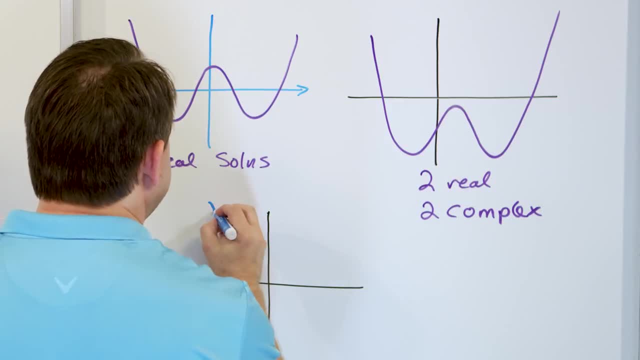 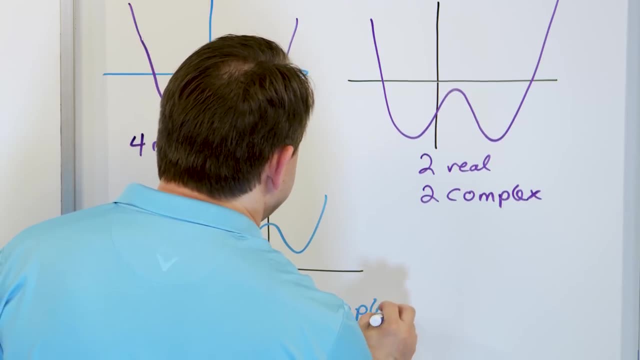 stuff. the final case: if the quartic actually goes down and up and down and up- but we never had any crossings at all- then we would have four real solutions, and then we have two real solutions or complex solutions. why have i gone through all of this stuff? the truth is, we're not going to learn. 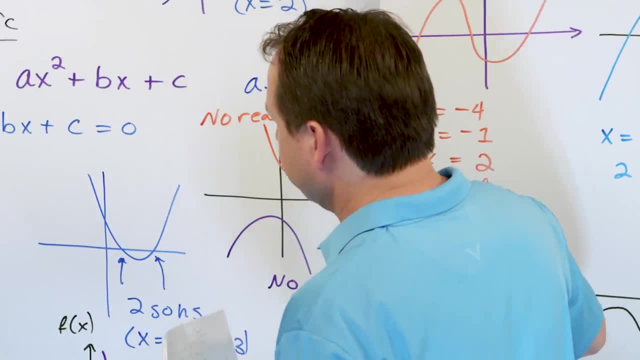 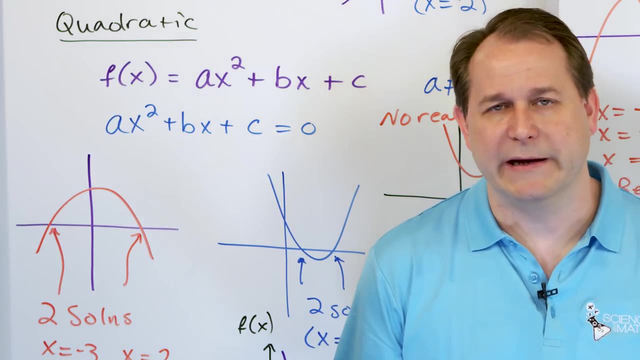 about quartic equations anytime soon. what we're really going to be doing is focusing on the quadratic equations, but oftentimes, i know, when i first learned this stuff, i didn't understand why we were doing it. why do we care? well, it turns out that solving polynomials, these are all different. 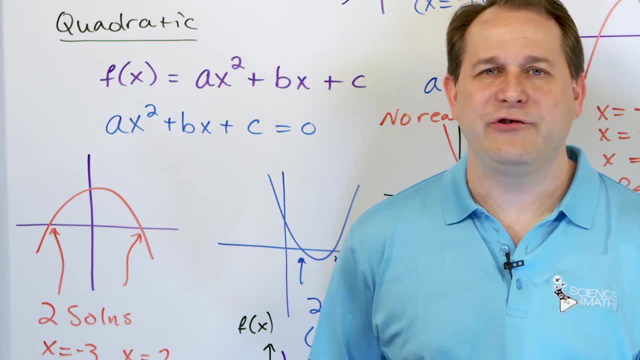 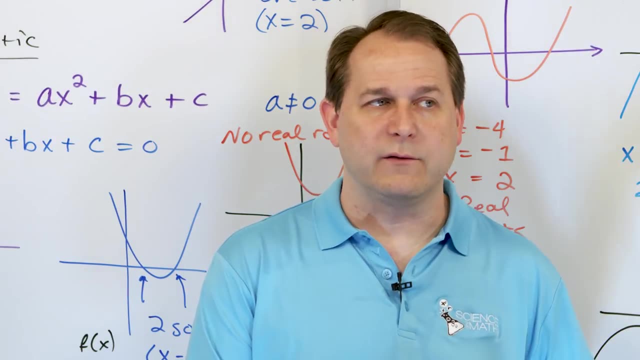 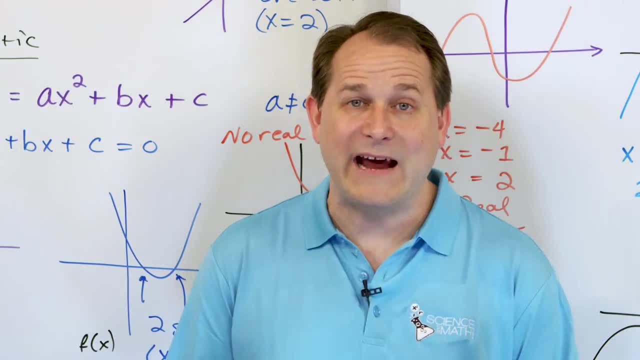 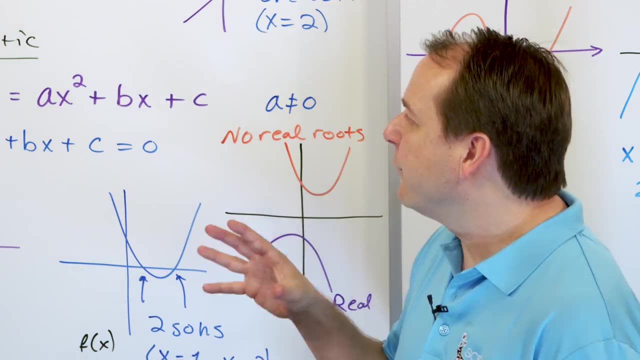 differential equations in calculus. oftentimes it boils down to solving polynomial equations as part of the solution process, so we have to crawl before we walk right. but this entire set of lessons is going to be focusing on the quadratic equations, so i want to give you an intuitive feel, because 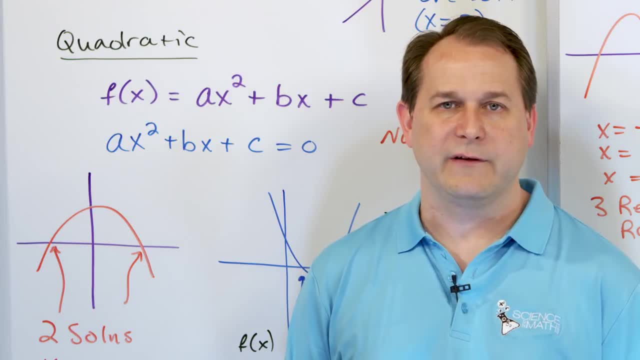 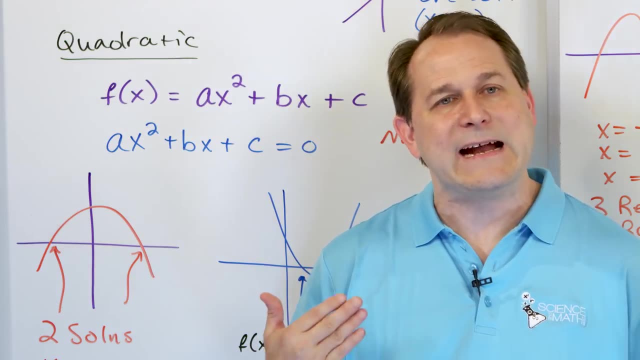 sometimes you're going to figure out that you you do have the two solutions, and sometimes you're going to find out that you have two solutions that are real and two solutions in other cases that are complex, and i never really understood when i learned this the first time. when do you have? 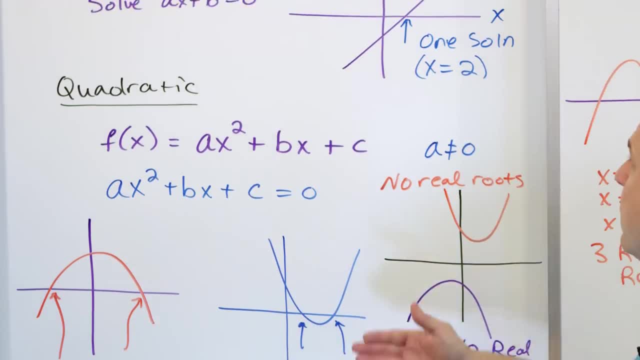 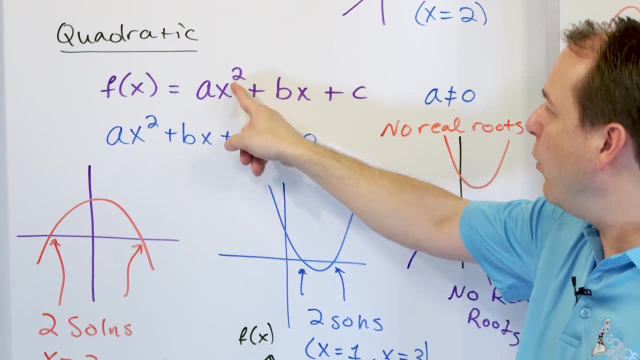 the real solutions and when do you have the complex solutions? this is what it boils down to. lines in general, cross in one location. you're going to have one solution because the highest power of x is a one. the quadratics are always going to have two solutions, but depending on where, 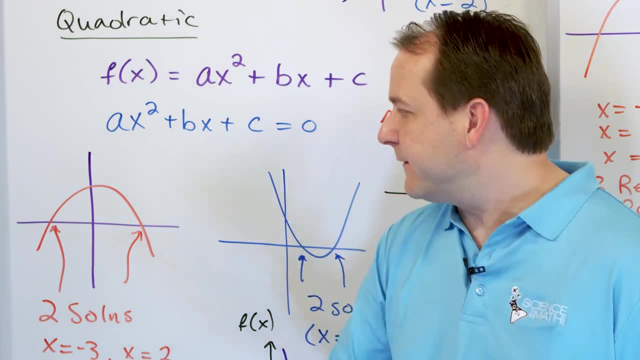 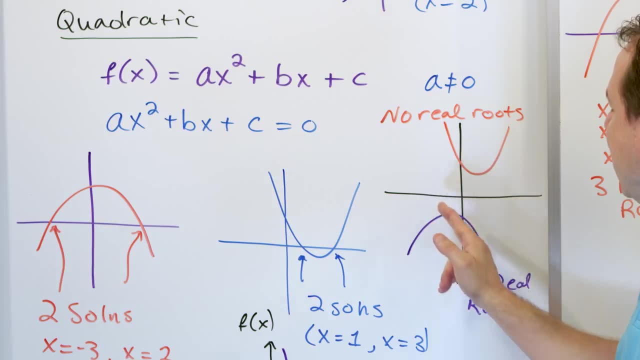 the graph is those two solutions can be both real or both complex. here we have two crossing points, so we have two real solutions. here we have two crossing points, so we have two real solutions. here we don't have any crossing points. all We still have to have two solutions. but they're both complex When you actually solve. 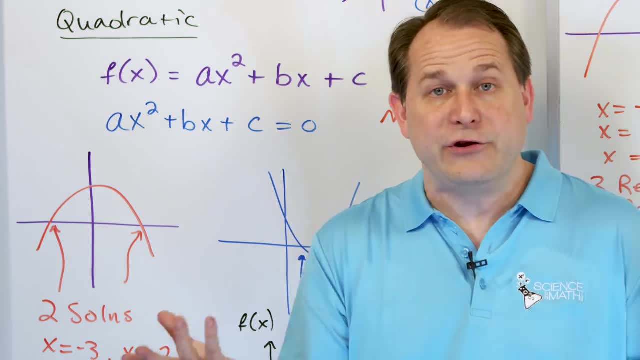 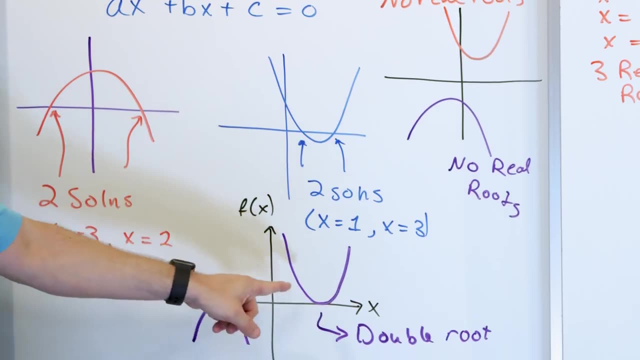 those polynomials that would give rise to these graphs. you'll find you're going to get with quadratic formula, which we'll learn soon. you're going to find that you get imaginary or complex solutions, And then we have the cases where the graph just kisses the axis, And we talked about 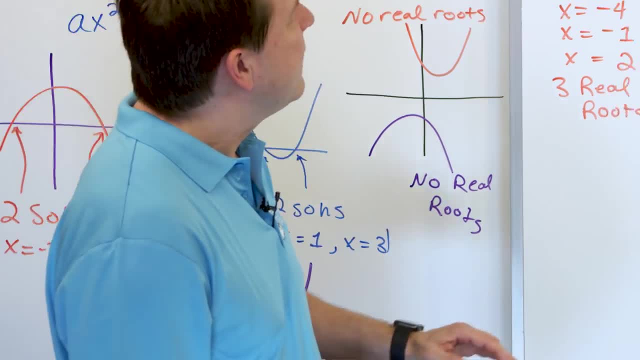 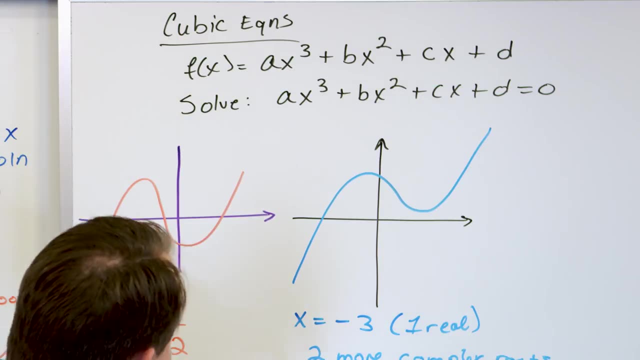 why these are double roots. They count as two roots as well, for a total of two. Then we have the cubic equations, which look like these snaky functions, And of course, remember, you can mirror, image or reverse them so that they go up and then kind of down like this: In general they'll cross. 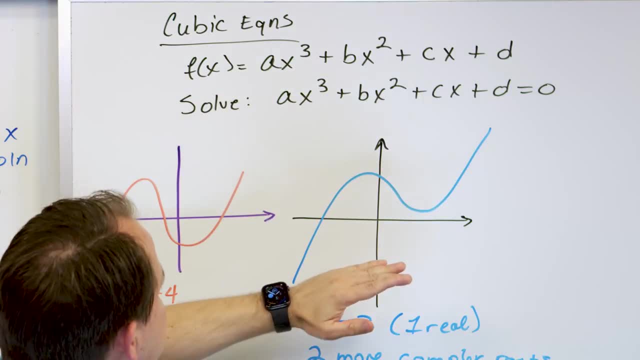 in three locations. three roots for a power of three. In this case it doesn't look like there's three roots really, but there is, because there's one real root, And then we have the two imaginary roots or complex roots that would make for a total of three Here. in this case, we'd have one real. 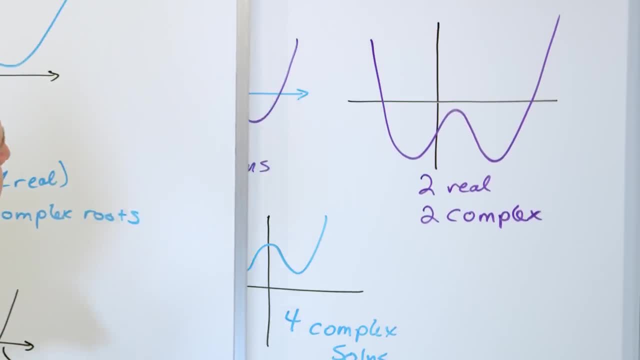 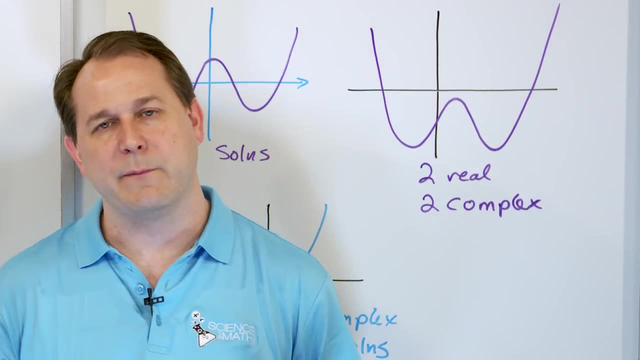 root, and then the other two would be imaginary or complex roots. And then we have the quartics where, in generally, we have four crossing points, but, depending on where the graph is, two of them might be real and two of them might be Complex. So that's why, when you're solving these equations- and we're going to be focusing on the 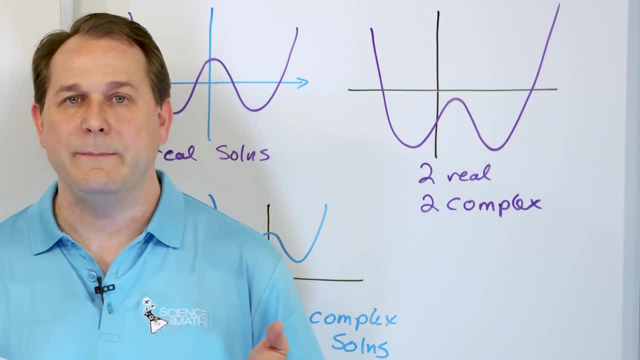 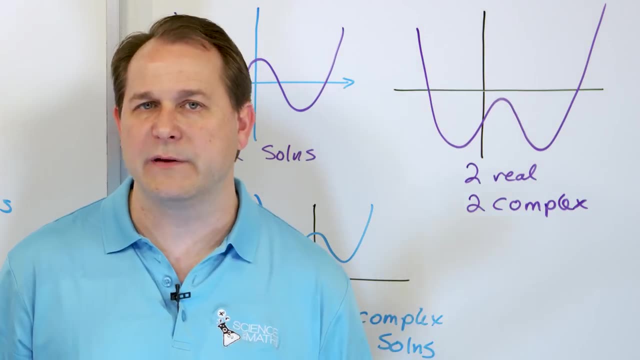 quadratics. sometimes you'll get real, Sometimes you get complex. What it means is if you were to graph those functions. that tells you what the graph really looks like. It tells you where the crossing points are, how many of them are there, And that's basically what it boils down to. 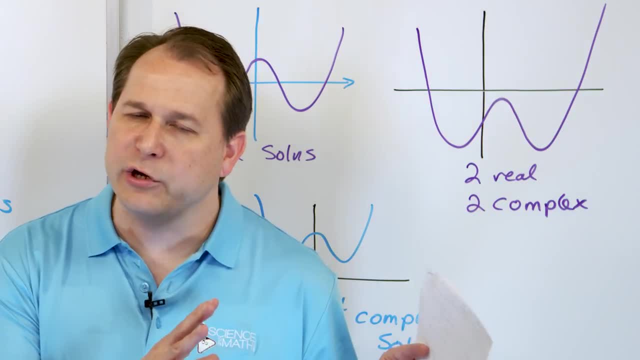 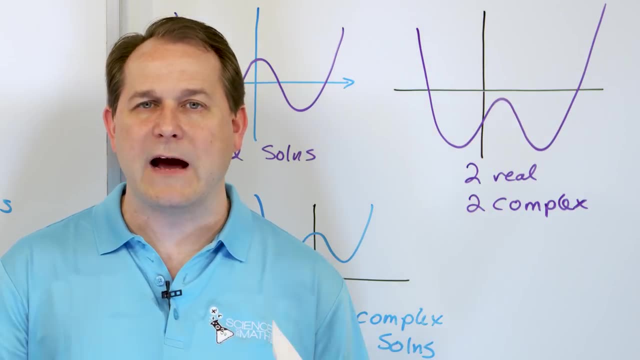 And that's all I want to really get into now. So what we're going to do is we're going to be learning how to solve quadratic equations with new methods that you haven't learned before. They're among the most important topics And types of equations that we're going to learn how to solve that have applications and 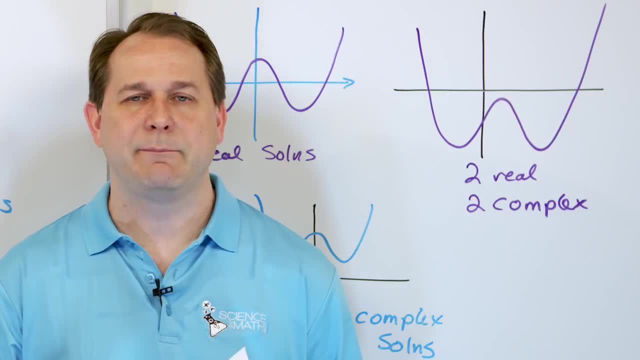 everything, So we're going to spend a lot of time on it. So follow me through the next batch of lessons and we'll be covering the solution methods for quadratic equations in great detail.